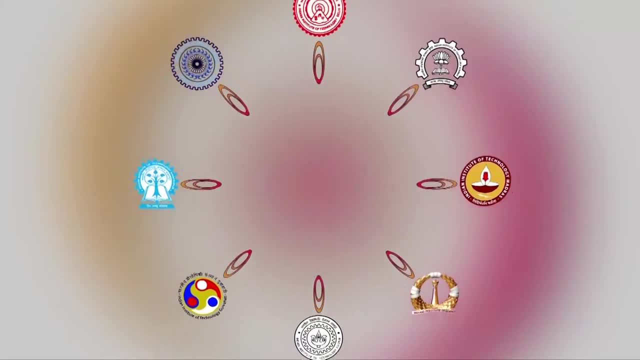 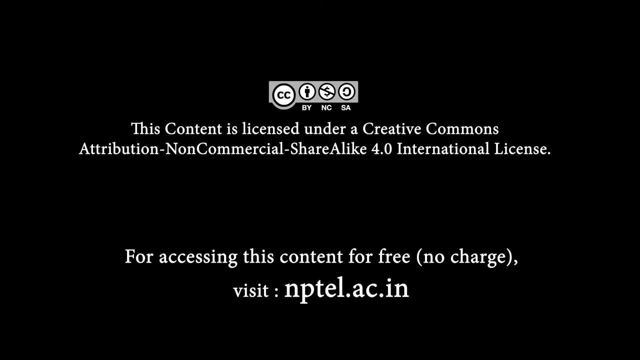 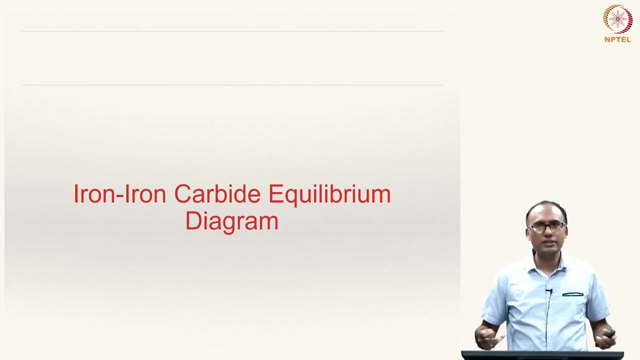 So now let us look at this iron-iron carbide equilibrium diagram, because it is very important system for us as mechanical engineers, because we will be dealing a lot with steel in general, and hence it is important to understand this particular phase diagram. So why are we studying? 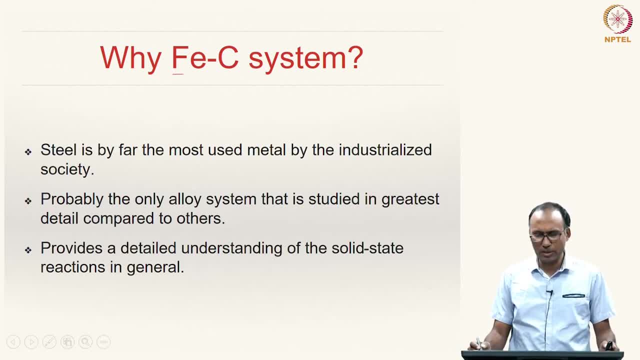 iron-carbon system, Because steel is by far the most used metal by the industrialized society and probably the only alloy system that is studied in greatest detail compared to any other alloy system. So you know a lot about this particular alloy system and 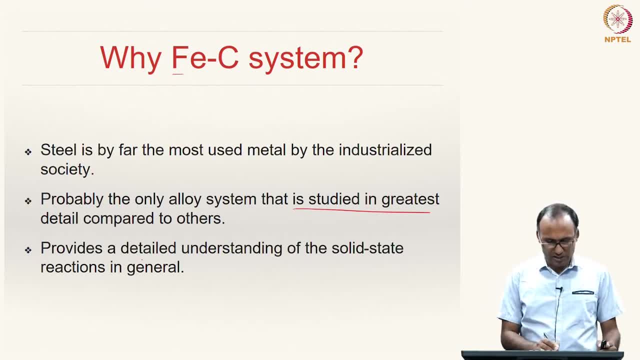 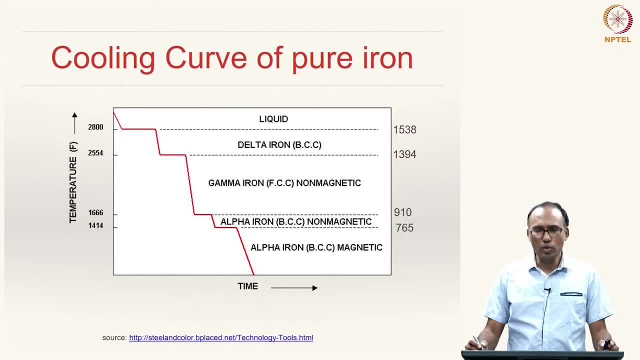 this iron-carbon phase diagram provides us a detailed understanding of the solid state reactions in general. So this is how the cooling curve of pure iron looks like. So this is the temperature shown in degree Fahrenheit. On this side it is shown in degree Celsius. So pure iron. 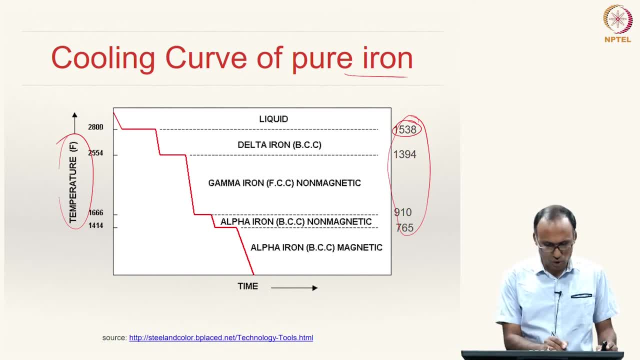 in the liquid state above 1538 degree Celsius or 2800 degree Fahrenheit, which is the melting temperature of steel, and when you cool it down at 2800 degree Celsius, the liquid transforms to solid state And at this position it is called delta iron, which has BCC crystal structure and at about 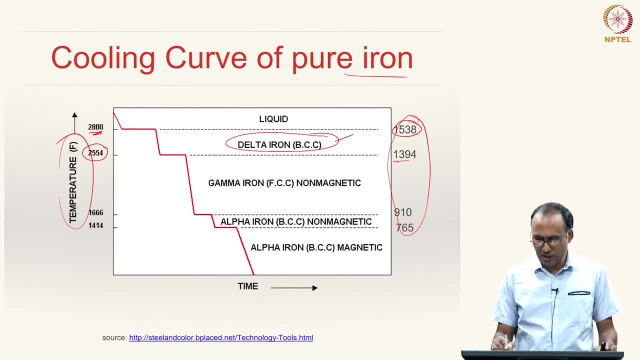 2554 Fahrenheit, or about 1400 degree Celsius, the delta iron undergoes an allotropic transformation and then…. So it is a solid state transformation and converts to gamma iron, which is FCC – phase centered cubic structure. So here you have an allotropic transformation. 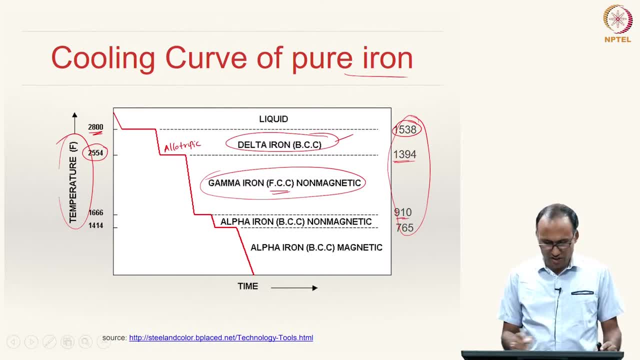 And then until 910 degree Celsius or 1670 degree Fahrenheit. the gamma iron is stable. but at that temperature, about 900 degree Celsius again, there is another allotropic transformation takes place, and then the gamma iron transforms to alpha iron right, And then alpha iron. 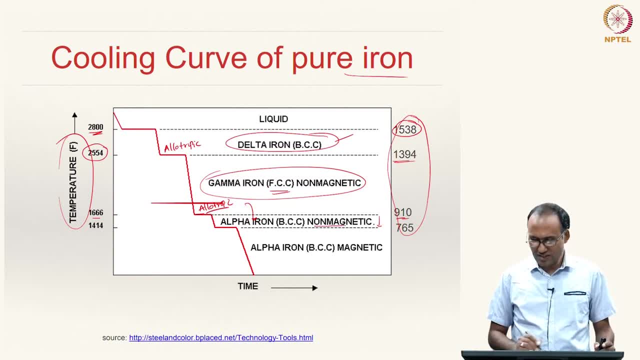 is going to be non-magnetic to begin with and until 765 degree Celsius, and below the 765 degree Celsius it regains its magnetic properties. It develops magnetic properties, right, But the crystal structure will still be BCC. 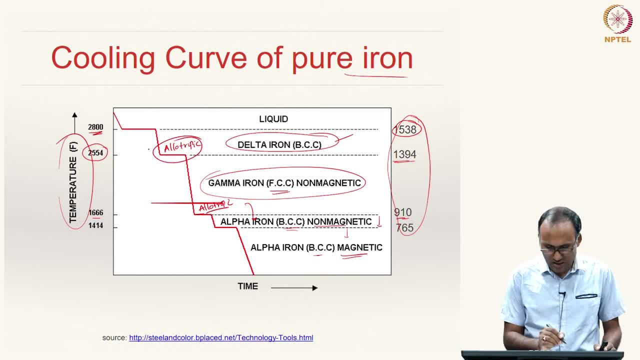 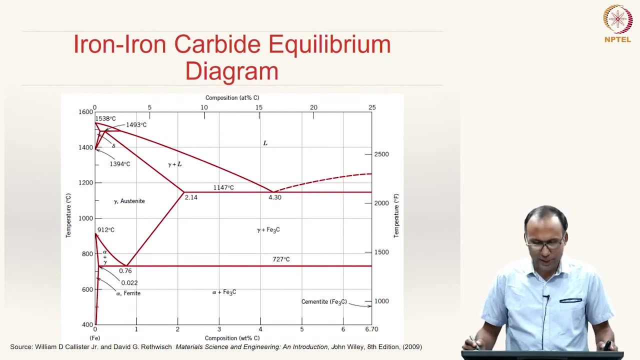 So for pure iron, as we have discussed, we have two allotropic changes, one from… When it is cooling down. one from delta iron to gamma iron, another one from gamma iron to alpha iron. Alright, So this is the typical iron-carbide equilibrium diagram. It is not iron-carbon. 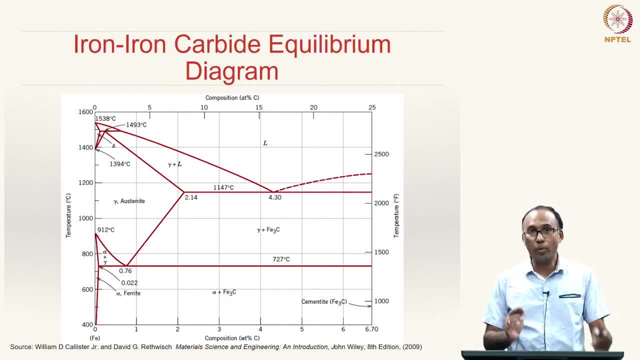 equilibrium diagram that we are showing here. It is a portion of iron-carbon equilibrium diagram And, as we have discussed in our 2nd class, we have seen that this diagram is basically type 4 alloys. whenever you had an intermediate solid solution, you can actually or intermediate: 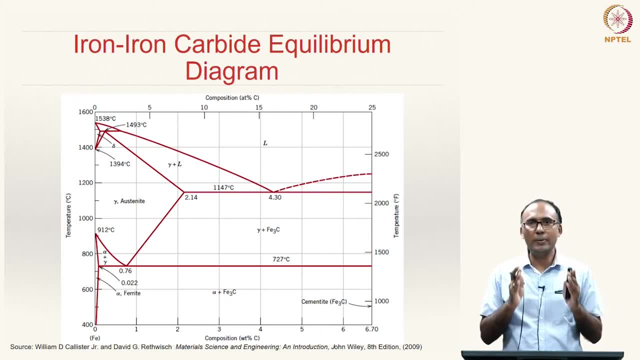 phase. you can actually see that portion as a independent phase diagram. same is the case here, actually, here we are seeing. on the left hand side you have a iron and this is the composition of carbon in weight percentage. on the top it is in atom percentage, the. 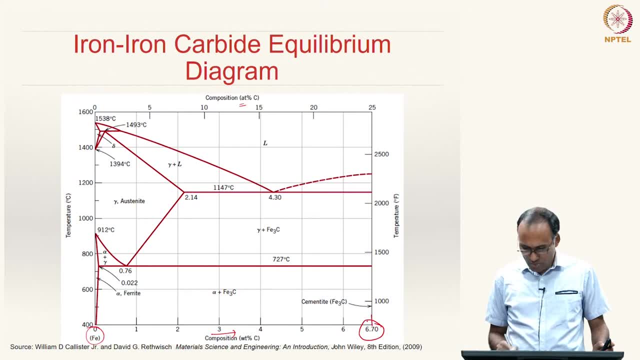 So 6.7 percent carbon. here you will have a special intermediate compound that is called cemented Fe 3 C, and right to that again you can have. So this is an specific compound and hence in between you can see this as a independent phase diagram, like as we have. 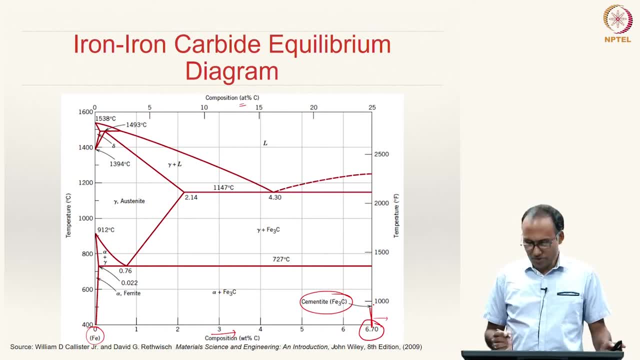 discussed in the type 4 alloys right. So the iron carbon is the carbon can actually the in the form of graphite can go up to 100 percent. but we are only interested in this iron iron carbide diagram because we will not use any iron carbon alloy beyond this carbon percentage, because that is going. 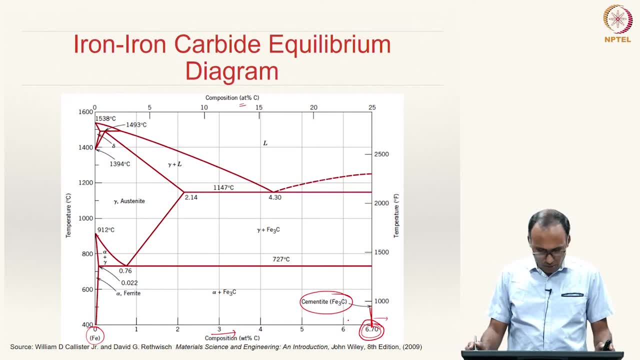 to be extremely brittle, all right. So for this phase diagram, on the left hand side you have iron and the right hand side you have Fe 3 C, all right, So let us identify some important points. So this is eutectic point. So liquid is transforming to two solids gamma. 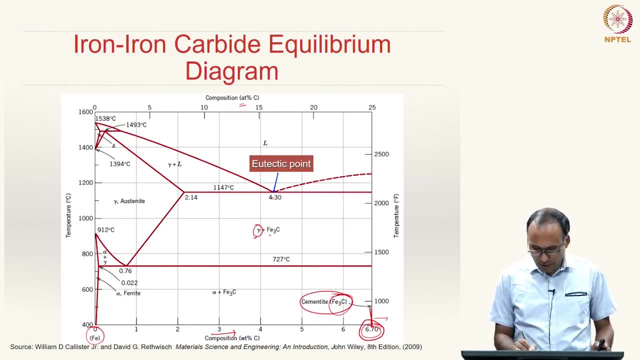 which is also called iron. So this is eutectic point and this is Fe 3 C. So another name for Fe 3 C is cementite. okay, So gamma is called austenite, alpha phase is called ferrite. this is your eutectic. 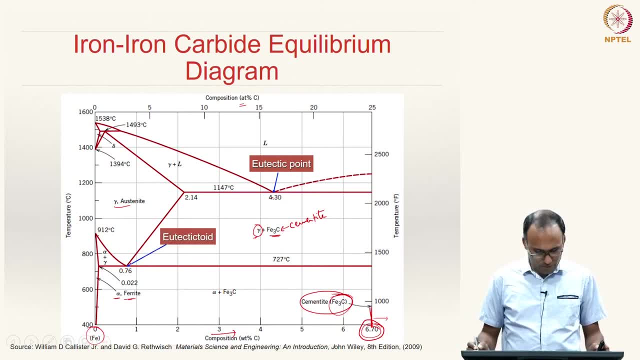 point, and that is our eutectoid point, where austenite transforms to ferrite and cementite. ferrite and cementite, So I will also call F plus C, ferrite and cementite, and this is our peritectic point, where liquid plus solid transform to another solid. So here this: 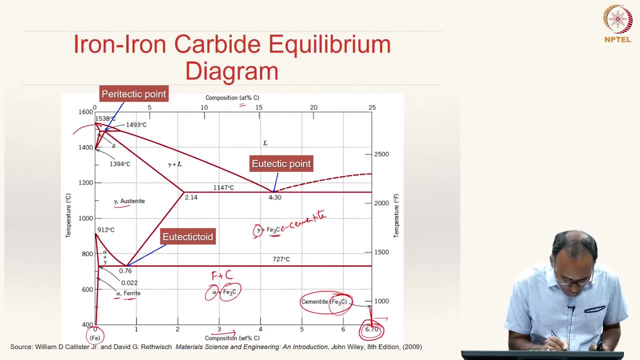 is our delta region. So this region, two phase region, liquid plus delta, upon cooling, will give you gamma. So that is our peritectic reaction point and it is important that we remember the compositions and the temperatures of these important reactions points. the eutectoid: 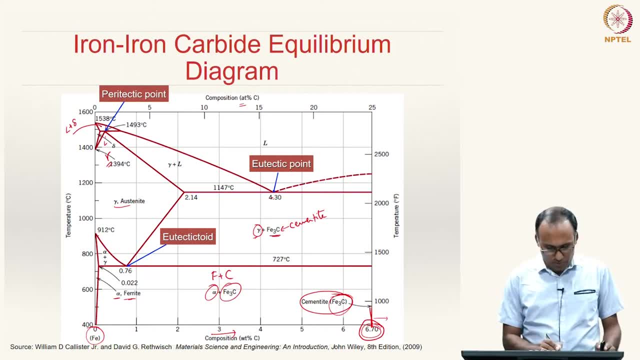 point. In some text books this number 0.76 can vary. in some text books it can. it is in this book it is written as 0.76. in some text books it is written as 0.78, 0.8.. So there may be slight. 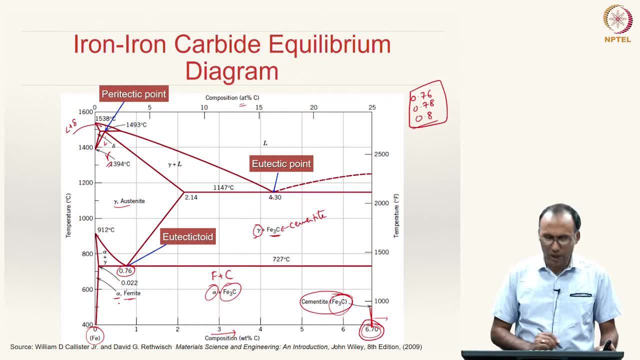 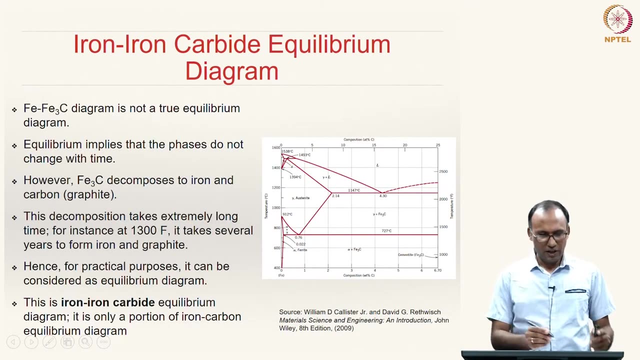 variation, but it is about 0.8. this percentage of carbon is about 0.8 and that is what is called eutectoid compound, eutectoid alloy. all right, We have heard that Fe, Fe 3 C diagram is not a true equilibrium diagram. why, whenever we 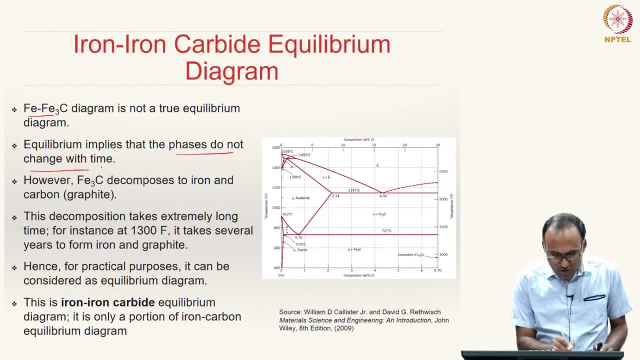 are saying equilibrium, it implies that the phases do not change with time. that means the phases that we are talking about should not change with time. if it is a true equilibrium diagram, However, the cementite or Fe 3 C decomposes to iron and carbon over time. 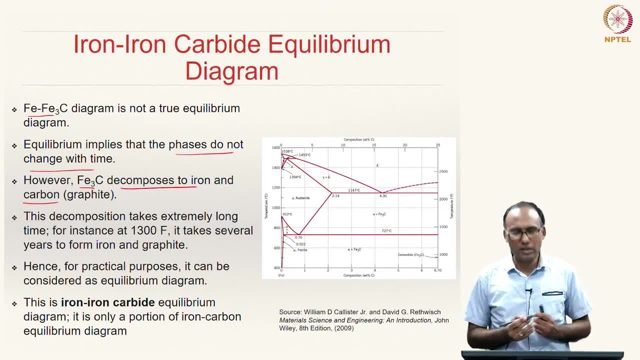 but this time can be very long time. but eventually it will decompose and hence, strictly speaking, we cannot call this iron iron carbon equilibrium diagram as true equilibrium diagram. However, as I mentioned, the decomposition takes extremely long time, several years, for instance at 1300. 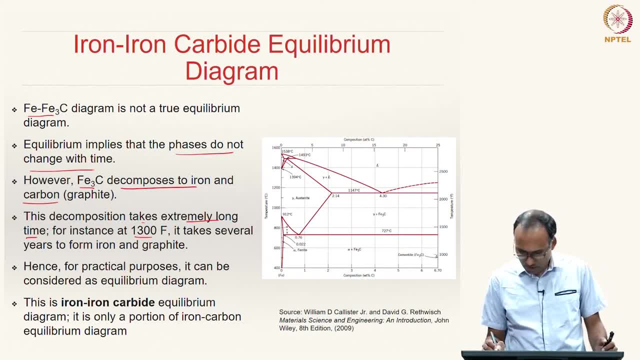 degree Fahrenheit. that is about this is 1000.. So that is about this temperature, this temperature. 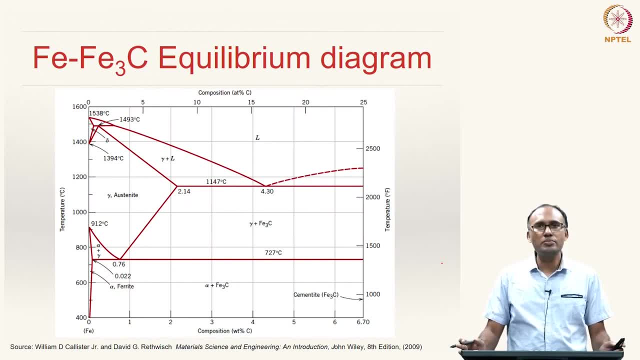 Alright. so all of you should be able to draw this diagram and you should be able to identify what are the compositions and the solubility. So, for instance, if you see this alpha ferrite has maximum solubility of 0.2.022. 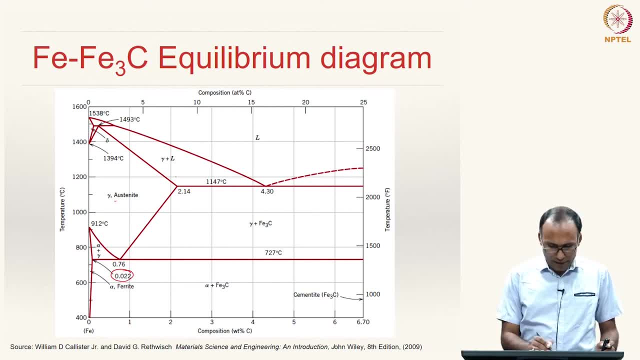 weight percentage of carbon here and gamma iron has 2.14 percent weight solubility of carbon in iron. So these solubility limits is something that way you should remember and you should be able to draw this diagram completely at the end of this course. 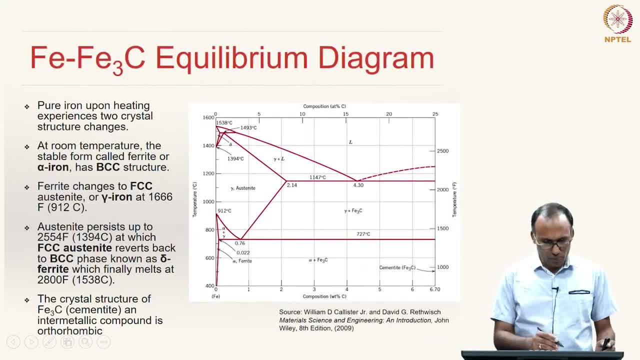 So, as we have discussed, so the pure iron upon heating experiences two crystal structure changes, as we have seen: one from delta iron to gamma iron and then from gamma iron to alpha iron, So at room temperature, the stable form called ferrite or alpha iron, which has 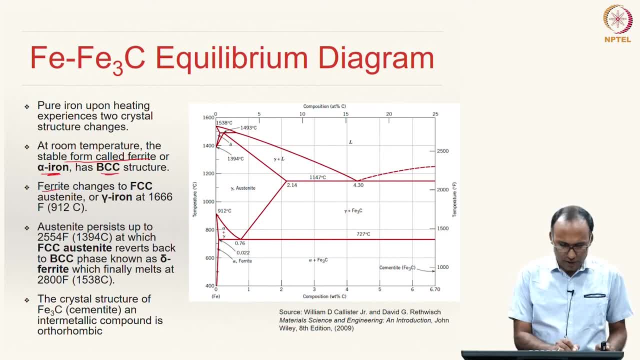 BCC structure and when you are heating it up, the ferrite changes to FCC structure and it is called austenite or gamma iron at about 1666 degree Fahrenheit or 912 degree Celsius. And austenite remains stable up to 2000- 1394 degree Celsius, or approximately 1400 degree. 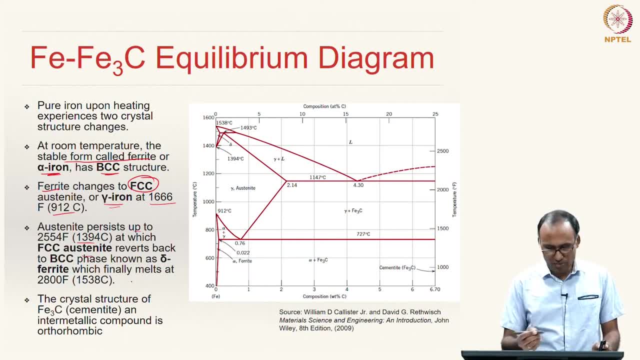 Celsius at which FCC austenite reverse back to BCC phase, but this BCC phase is known as delta ferrite and which finally melts at 2800 degree Fahrenheit. So we have seen two phase transformations: alpha iron to gamma iron and gamma iron to delta iron. So the crystal. 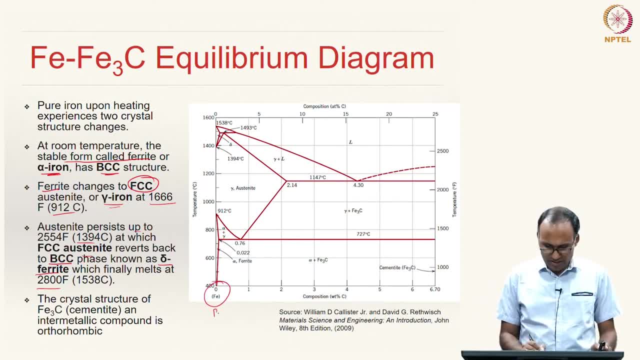 structure of iron at room temperature is BCC, and what is the crystal structure of Fe 3 C? The crystal structure of Fe 3 C, which is an intermetallic compound, is orthorhombic. Now, the crystal structures of Fe 3 C are of different types. We have already discussed. 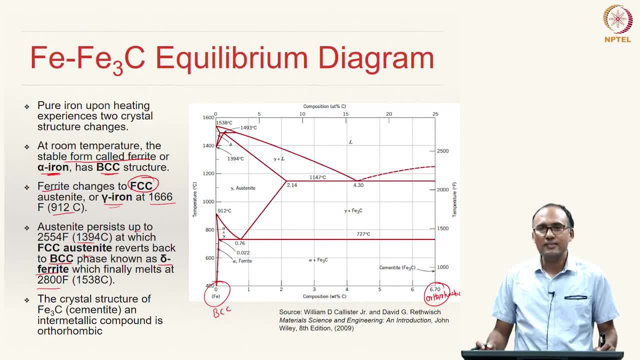 the size of the carbon atom is relatively smaller compared to the size of iron atom, and hence that is one thing. and the second thing is their crystal structures are not the same. So Fe 3, C and the carbon crystal structure is diamond structure and hence their 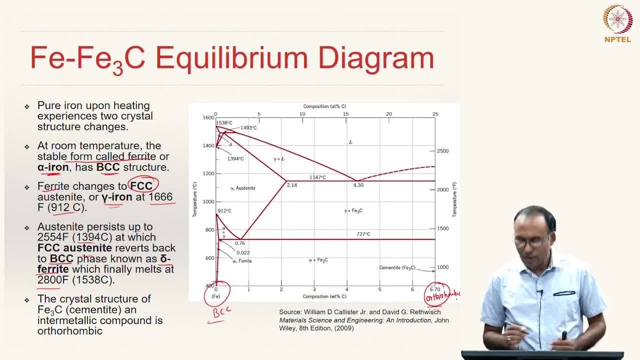 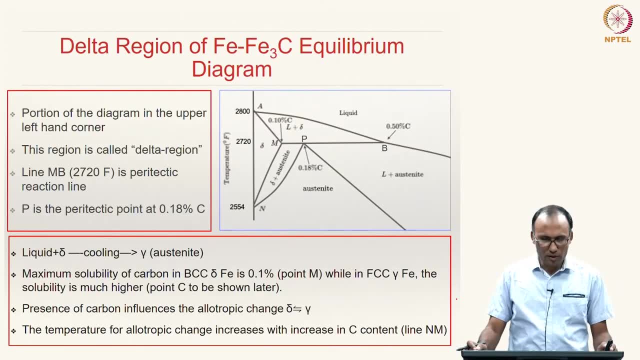 crystal structures are not the same. even if you see Fe and Fe 3 C, they have different crystal structures, Hence they will only form an interstitial solid solution. all right, So now let us look at each of these regions, important regions in FEFE3C diagram. So this is what this region 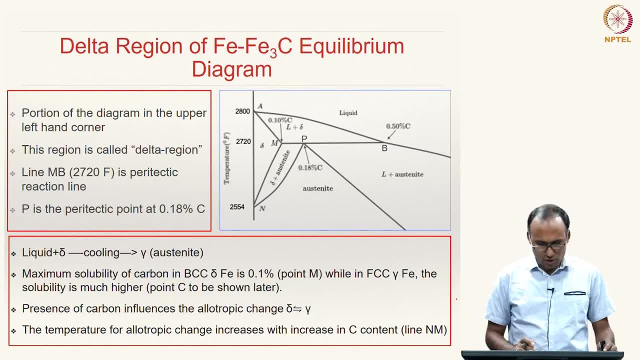 is called delta region, where the delta iron is stable. So this is the portion upper left hand portion of the phase diagram, this area that we are zooming in and then trying to see what is happening there. So here you have the position m, p, b and that is our pyritectic. 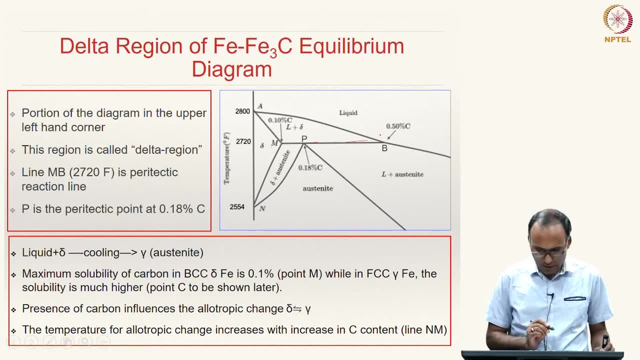 line. So the pyritectic reaction takes place along that line. Line m, b is called pyritectic reaction line and p is the pyritectic point at 0.18 percent carbon. So the pyritectic 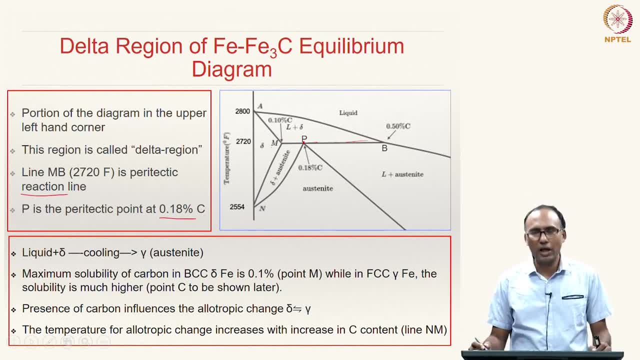 point. so if you are talking about a pyritectic alloy, that is 0.18 percent carbon. So what is the reaction that is taking place here At the point p? liquid plus delta transforming to austenite or gamma iron. So liquid plus. 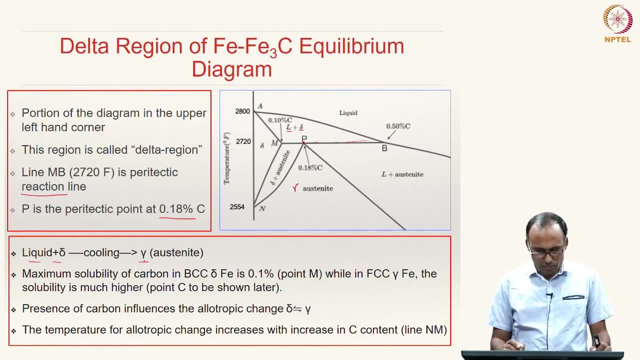 delta upon cooling gives you gamma. So the maximum solubility of carbon in BCC delta iron is about 0.1 percent. that is this right. So this is the maximum solubility. you cannot have more than 0.1 percent carbon in BCC delta iron at point m, while in FCC we would see. 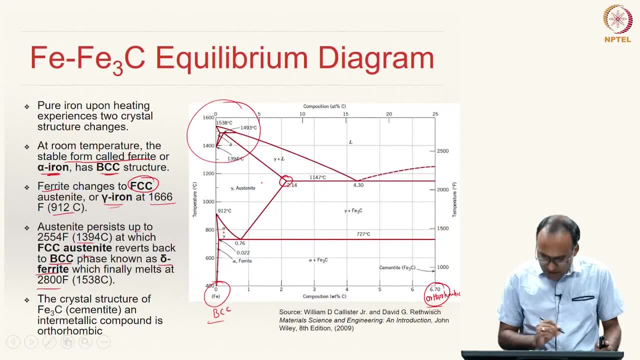 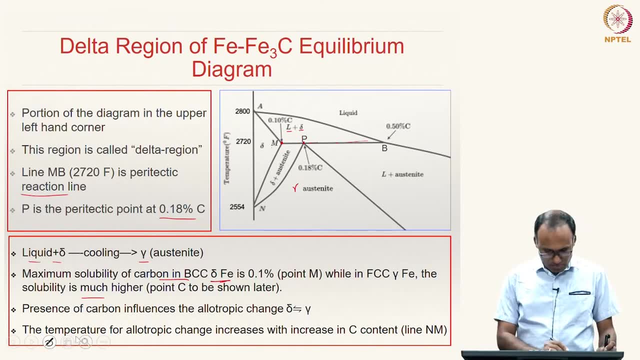 the solubility is much higher. We can see that then FCC: the solubility is 2.14 percent as compared to 0.1 percent in the BCC delta iron. So the temperature for this allotropic changes increases with increase in carbon content. 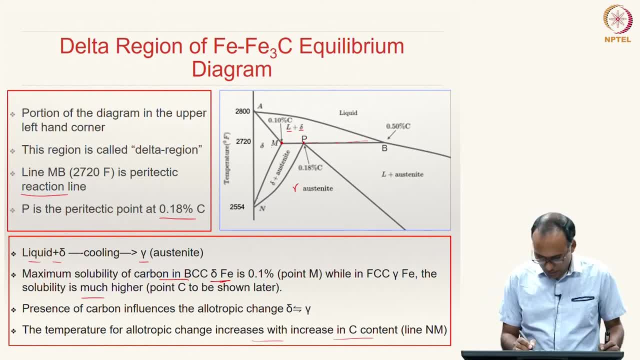 right. So we can see that here. pure iron converts from gamma iron to austenite, sorry, gamma iron to delta iron at 2554 degree Celsius. but if you are at higher temperature, for instance higher carbon contents of somewhere here, then your complete transformation to delta. 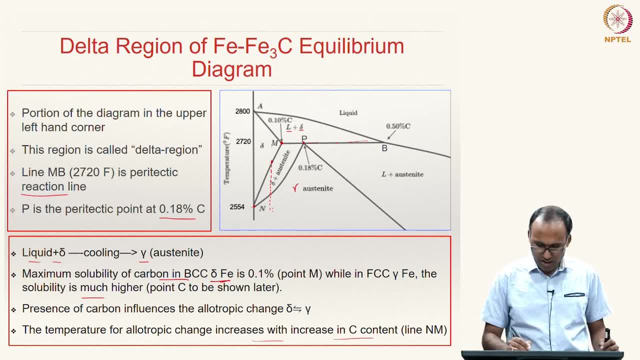 iron. it starts here and it ends here. So austenite starts transforming to delta iron here, ends transforming to delta iron here. That means it happens at a higher temperature than for the system which has lower carbon content. So that means the temperature for. 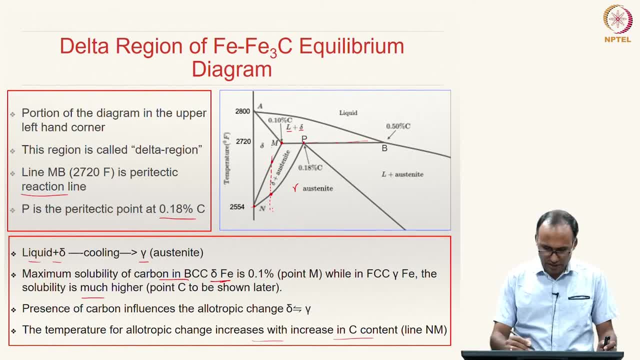 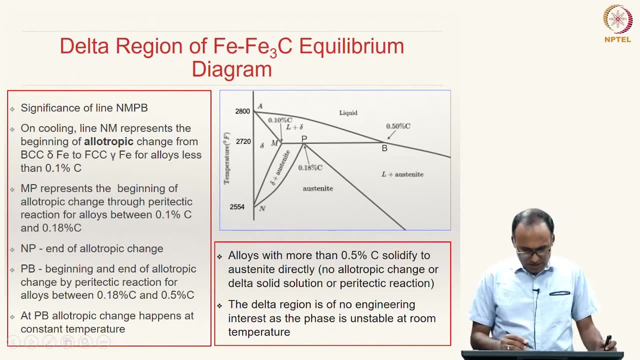 allotropic change increases with increase in carbon content. that is described by this line nm. So what is the significance of line nmpb? So, on cooling the line nm, when you are cooling down, the line nm represents the beginning of allotropic change and the line np sort. 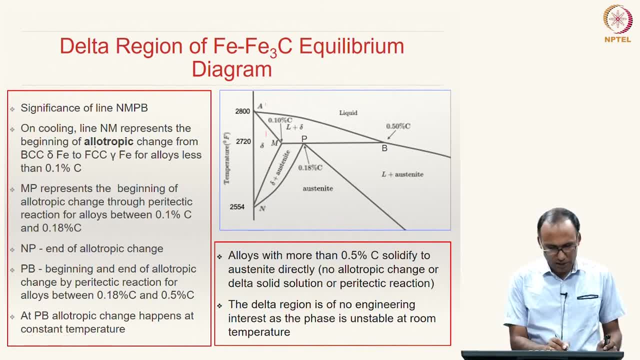 of represents the end of allotropic change, right? So beginning of allotropic change from BCC- delta iron to FCC- gamma iron for alloys less than 0.1 percent carbon. This is the starting allotropic change starting point for alloys less than 0.1 percent carbon and m p. this 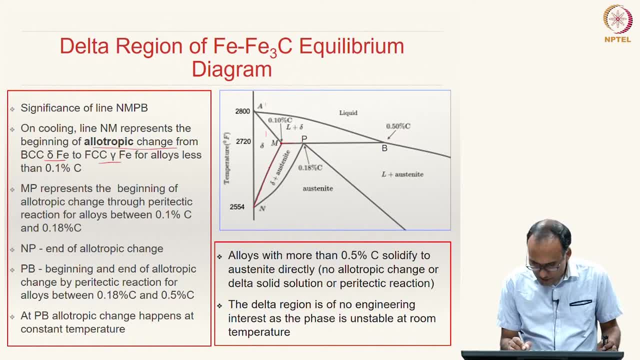 portion represents the beginning of allotropic change. right delta transforms to austenite through, not through, periodic reaction, So it the beginning of this. delta plus liquid plus delta is transforming to austenite is through periodic reaction for alloys between 0.1 percent and 0.18 percent and n? p of course represents the end of allotropic change and 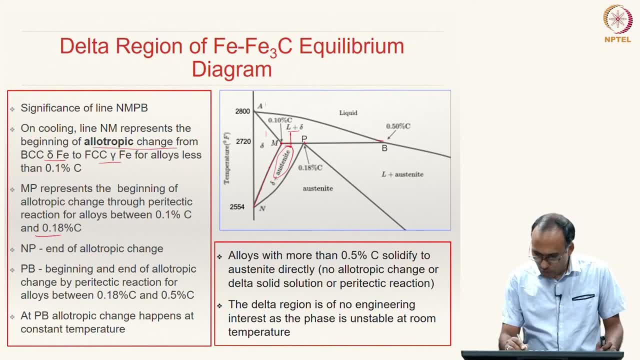 the line p b is beginning and end of allotropic change, because the below that you only have here you have liquid plus delta. this is liquid plus austenite. So all the reaction that will take place is some amount of liquid plus delta and then the end of allotropic change. plus delta would be converted to austenite and still some amount of liquid remains. So this is the beginning and end of allotropic change. here the allotropic change happens at constant temperature, whereas left to p, allotropic change happens over a range of. 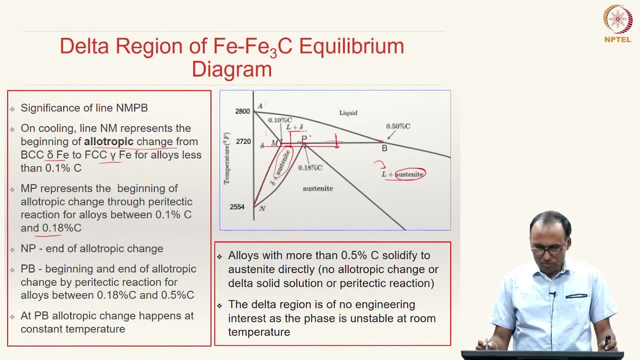 temperature and for alloys with more than 0.5 percent carbon, you do not see the formation of delta iron. So the delta iron is not necessarily always a stable form of carbon. So delta phase, because it depends on the carbon content. if the carbon content is greater than 0.5 percent. 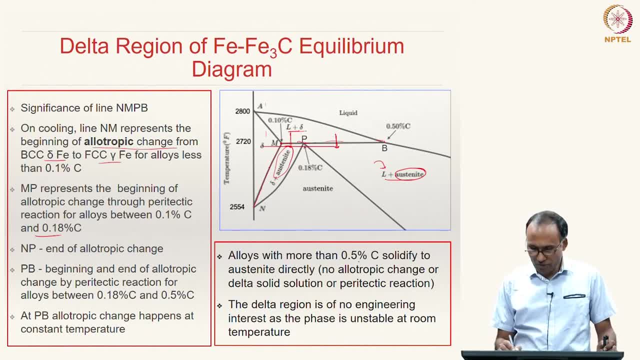 you will not have delta phase at all. So 0.5 percent carbon solidify directly to austenite. they will not go through allotropic change. So the delta iron is only stable in the portion where the carbon content is less than 0.5 percent. and as, however, this the region of 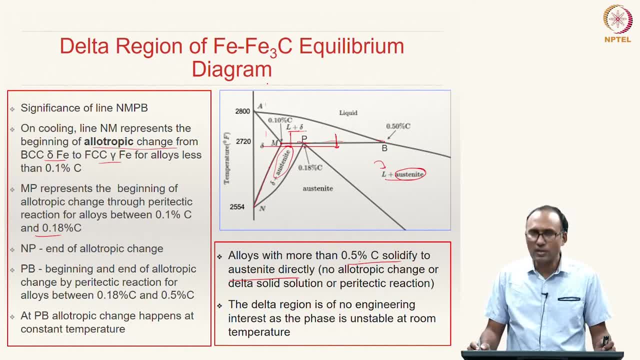 delta, the delta iron or delta region is usually of not great engineering significance because this phase is constant. So the delta phase is seen as a constant phase. So the delta phase is unstable at room temperature. For plain carbon steels it is not stable at room. 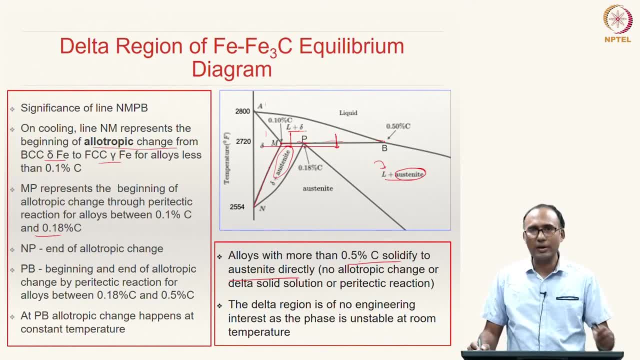 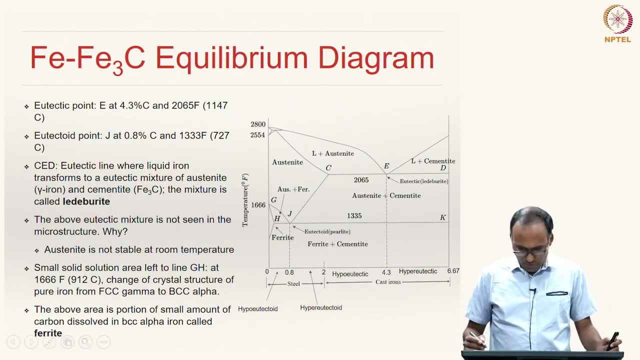 temperature, and hence not so much attention is usually paid to delta phase. So now let me…. We have redrawn this iron carbon-nucleotide diagram, and then E is our eutectic point and J is our eutectoid point, and C represents the maximum solubility of. 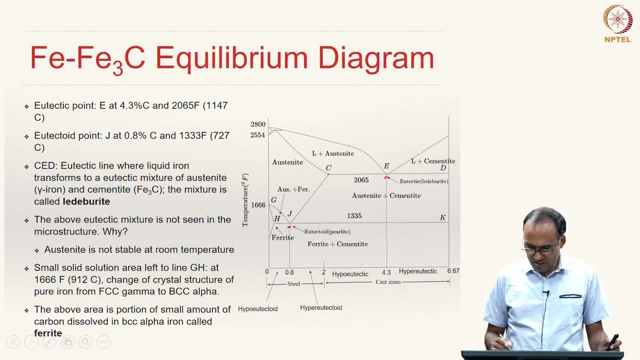 carbon in austenite and other two-phase regions are represented. So the eutectoid… So the eutectic mixture, the liquid, when it is going through eutectic reaction, it will form austenite and cementite. right, It will form a eutectic mixture of austenite and cementite. 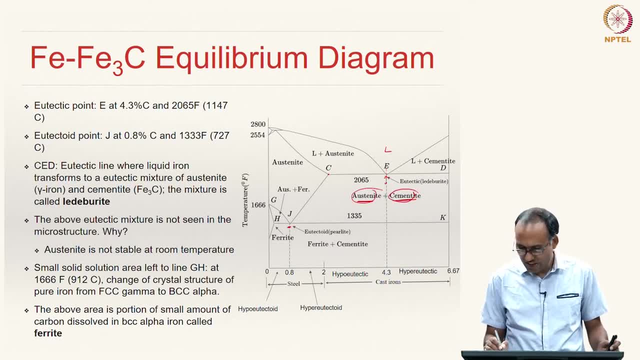 The eutectic mixture of austenite and cementite is having a special name called leadbrite And similarly, at eutectoid reaction, austenite is transforming to ferrite and cementite, So this will be eutectoid mixture of ferrite. 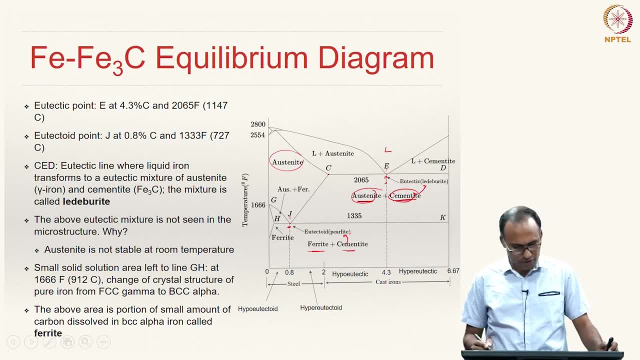 and cementite that has a special name called perlite. You have to remember these names. So the C line, CED, represents eutectic line, which gives you the microstructure leadbrite, and the line HK represents our eutectoid reaction, which gives us the microstructure perlite. 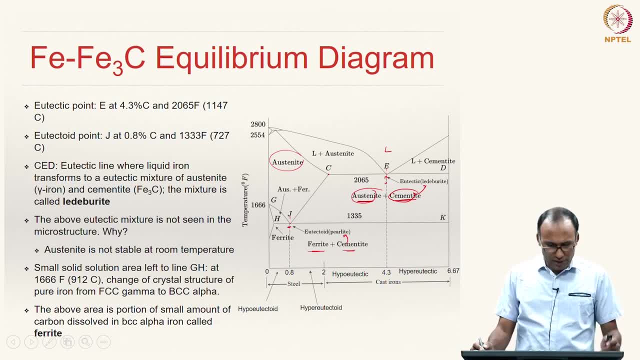 Thank you. So usually in steels the eutectic mixture is not seen, because even though you have formed the eutectic mixture of austenite and cementite, the leadbrite, it will again go through at room temperature, it will again go through eutectoid reaction and eventually 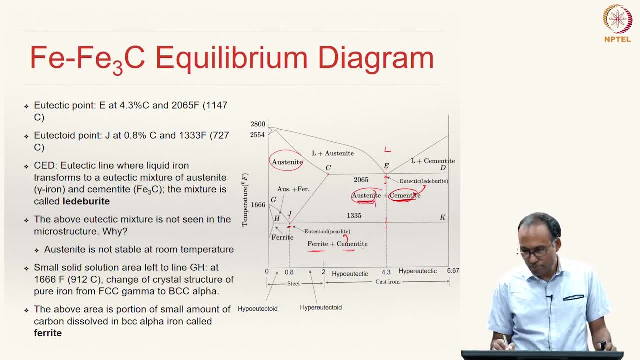 you will only have ferrite and cementite, because austenite is not stable below this temperature. right And small solid solution area left to join. you have a very small solid solution area left to join And when you have a small solid solution area left to join. 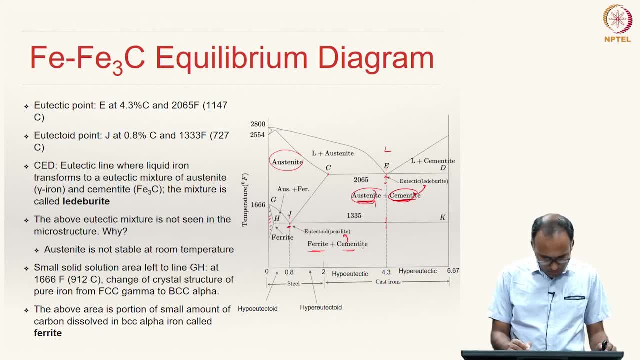 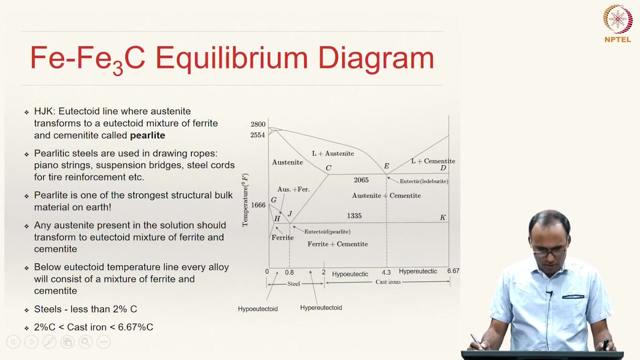 to g, h, that this position. you will have a change of crystal structure, as we have discussed, from gamma to alpha, and then this is what is called ferrite, which is B C, C, having B C, C microstructure right. So this should be our, this is our ferrite, so all right. 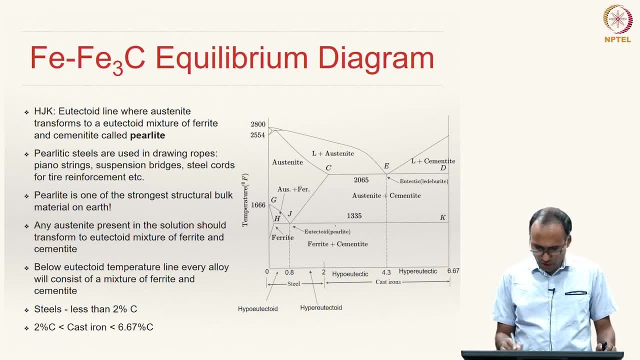 So the line h, j, k- I have already mentioned that- is a eutectoid line. the mixture is called perlite. the perlite steels are used usually in drawing process, drawing ropes. the applications are piano strings, suspension bridges, steel cords and for tyre reinforcement and so on. 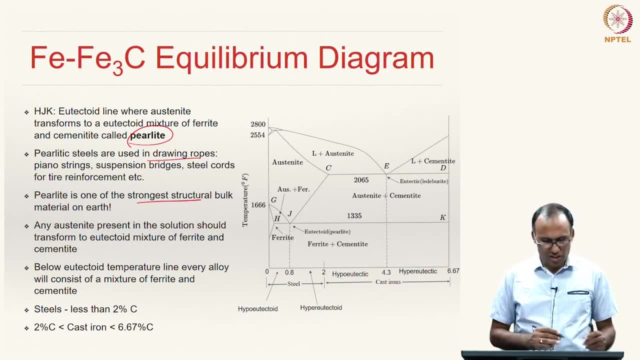 and perlite is one of the strongest structural bulk material that is known for us, and any austenite present in So in the solution should transform to eutectoid mixture of ferrite and cementite because austenite is not stable below this 1335 degree Celsius temperature, Fahrenheit temperature, right and 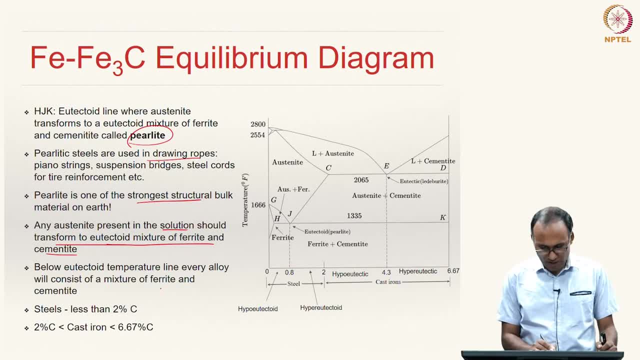 so the below eutectoid temperature line. every alloy will consist of mixture of ferrite and cementite. and here you see that the 0.8 percent carbon is the eutectoid composition. left to that it is called hypo eutectoid alloys and right to that it is called hyper eutectoid. 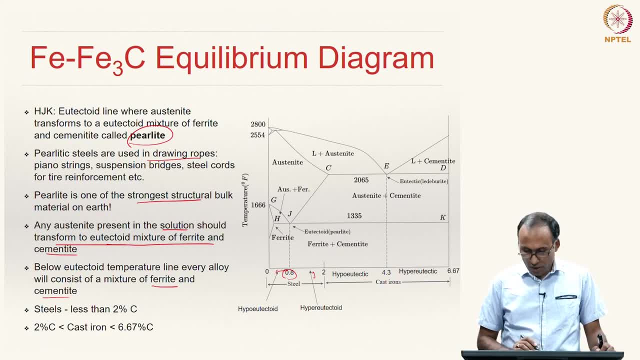 alloys right, and usually steels are the iron carbon alloys which have a carbon percentage less than 2 percent are considered steels. So whenever we are calling steel, it is an iron carbon alloy with carbon percentage less than 2 percent. So that is why only up to 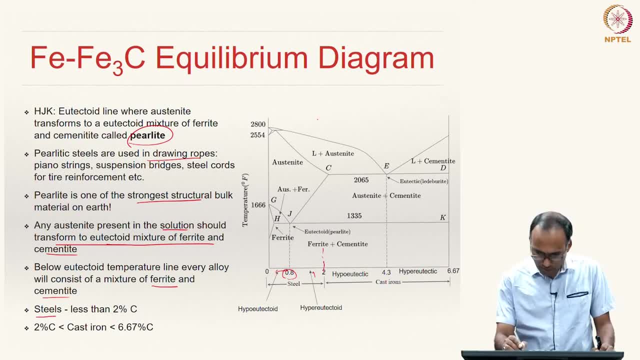 here, right? So this portion is only considered steel. So this portion is only considered steels and after, if the percentage of carbon is greater than 2 percent, and between 2 and 6.67 percent, and then they are called cast irons. all right, 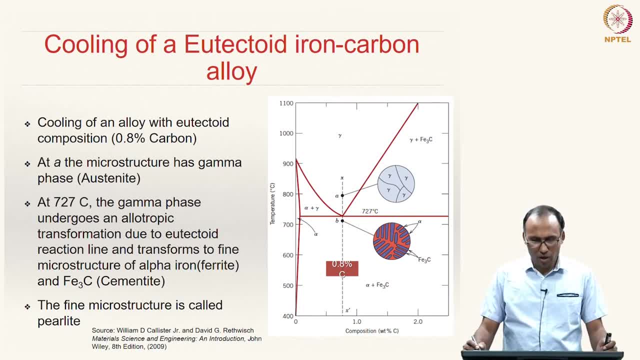 So now let us look at the microstructure evolution of a eutectoid iron carbon alloy. So eutectoid percentage is about 0.8 percent carbon. as we have discussed, it can be 0.76 to 0.8, but 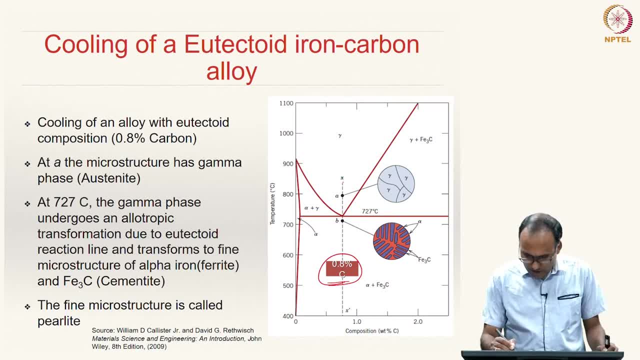 he in this class. let us say it is 0.8 percent carbon, So here it is gamma iron. So at A it will be gamma iron and the moment it reaches point B it will go through eutectoid reaction. that means the gamma will transform to two solids. 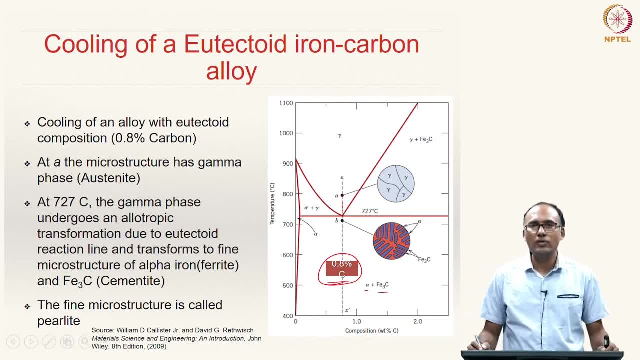 alpha and Fe 3 C. but it will not give some generic microstructure, but it will have alternate layers of ferrite and cementite. So that is like this: So the red ones are our ferrite and the blue ones are our cementite. So you will have alternate layers of ferrite and 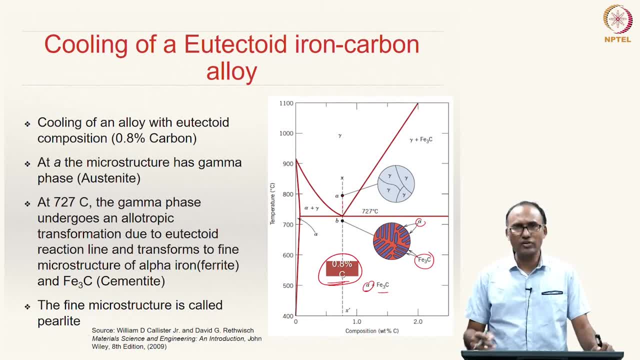 cementite, just like the eutectic microstructure. So there is complex material되o for eutectoid, a special name called ferrite. So this fine microstructure that we have discussed in the previous lectures, And this fine microstructure is called perrylite, So this is a having a special name called perrylite. 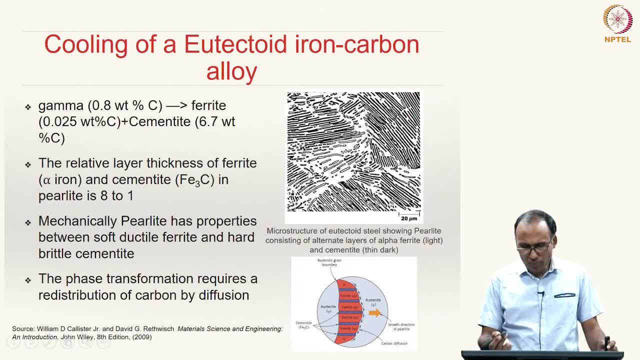 Perrylite is a eutectoid mixture- ferrylite and cementite- So under the microscope this look something like this. This micrograph represents the Robert SOLIXBrown medida three MiG�T 13 microstructure of eutectoidvention steel. when we say usted steel, that means it is 0.8 percent. 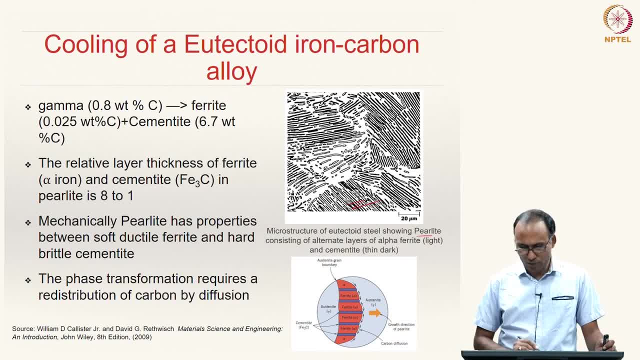 carbon. steel is 0.8 percent carbon, And then that that is represent不是 Украї information in dring with odorsliderist. However, while this nice microstructure, or this great microstructure that is called a pearlitic microstructure, So the relative layer thickness of ferrite. 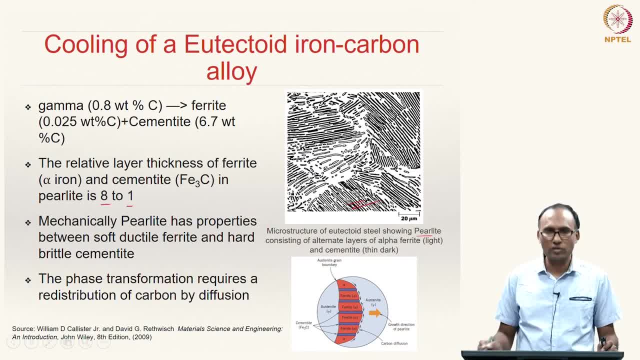 and cementite in pearlite is about 8 is to 1. So that means the layer thickness of ferrite is larger than the layer thickness of cementite. So the mechanically the pearlite has properties between soft ductile ferrite and hard brittle cementite. So it will have properties between 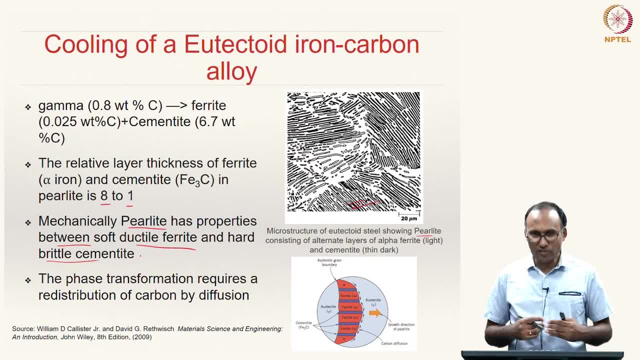 ferrite and cementite and the phase transformation, as we have discussed, requires a redistribution of carbon by diffusion and, as we have discussed in the case of eutectic reaction, why they have alternate layer formation rather than separate islands of this ferrite and cementite. 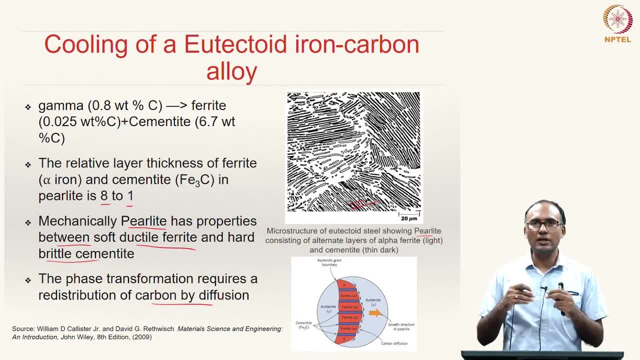 That is because if you have alternate layers of ferrite and cementite, the requirement for atomic diffusion is less, So that make diffusion can happen only over short distances, as we can see in this figure here. all right, So now all the alloy compositions left to eutectoid. 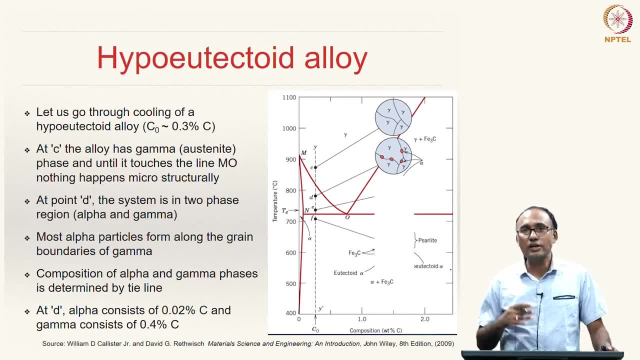 composition are called hypo eutectoid alloys. all the alloys right to the eutectoid composition are called hyper eutectoid alloys. So all the steels which have less than 0.8 percent carbon are called hypo eutectoid steels. all the steels which have carbon percentage greater. 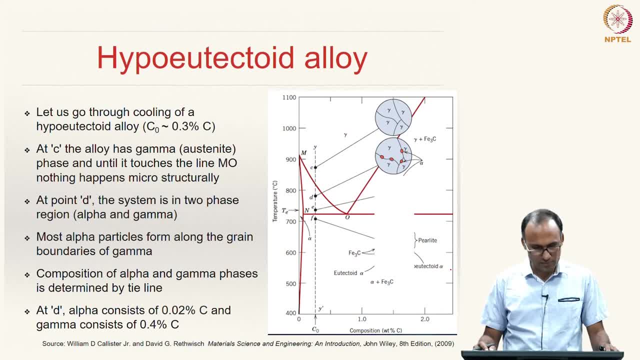 than 0.8 percent carbon are called hyper eutectoid steels, right? So now let us look at the microstructure revolution in the case of a hypo eutectoid steel. So here we are. so this is our eutectoid composition. So let us go through the cooling of a hypo. 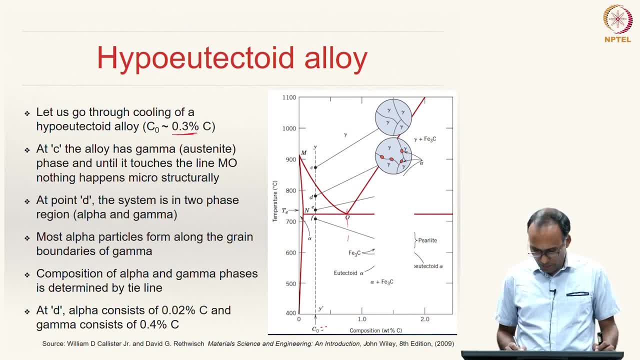 eutectoid alloy, whose composition C naught equal to 0.3 percent carbon. So at point C you have gamma, iron, austenite, and, as this point, as you are cooling down the, until the temperature reaches this point, nothing happens. everything will be gamma. but as soon as it, 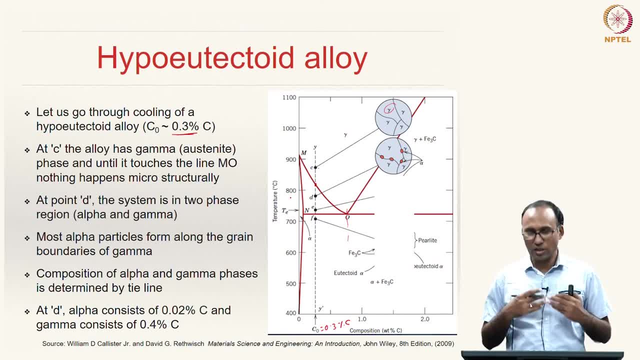 starts hitting this M O line, this the transformation from gamma to ferrite- starts happening. right, because this is alpha. So this is a two phase region. when you draw a tie line here, and this is our gamma phase and this is our alpha phase, So you will have: 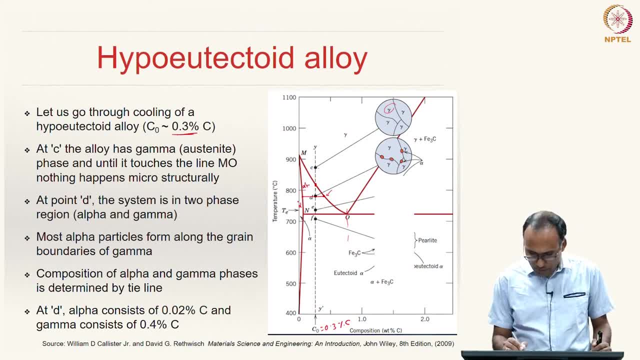 have a two-phase region which is alpha plus gamma. right At point D the system is in two-phase region- alpha and gamma- and most alpha particles form along the grain boundaries of gamma. So here you can see that gamma and around the grain boundaries you are forming. 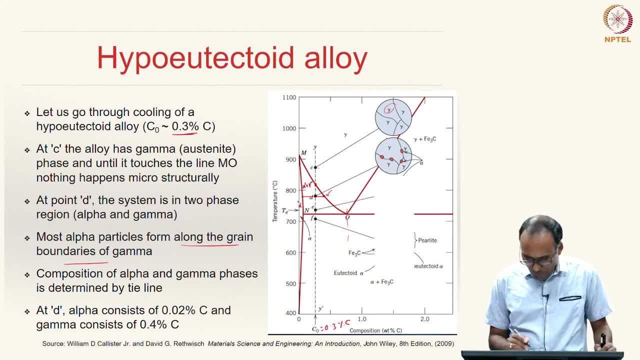 the alpha particles. And you can also find out the compositions of alpha and gamma by drawing a tie line and draw the verticals and then you will find out what is the composition of gamma. And if you draw the vertical here and then you will know what is the composition, 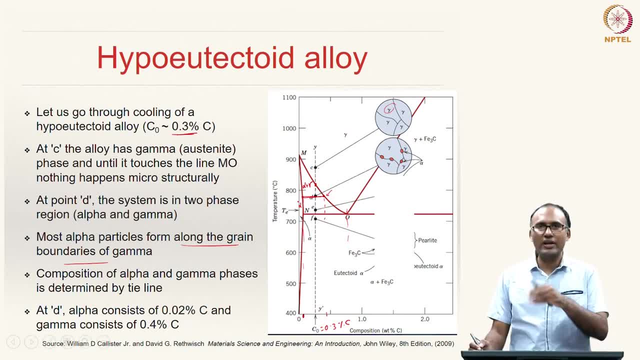 of alpha, or what is the composition of gamma? When I say alpha, it is ferrite, When I say gamma, it is austenite. So we can see that at point D, the alpha is having a composition of 0.02 percent carbon and gamma has about 0.4 percent carbon. This is 0.5.. So, and hence, 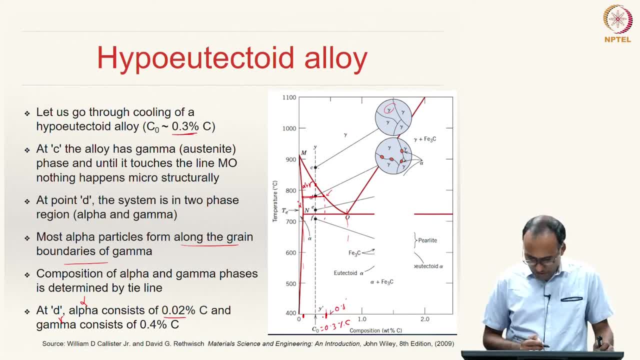 this is about 0.4 percent carbon, And then you can also calculate the weight fractions right By using the liver rule: 0.02 and 0.4,. all right, So if you further cool it down as 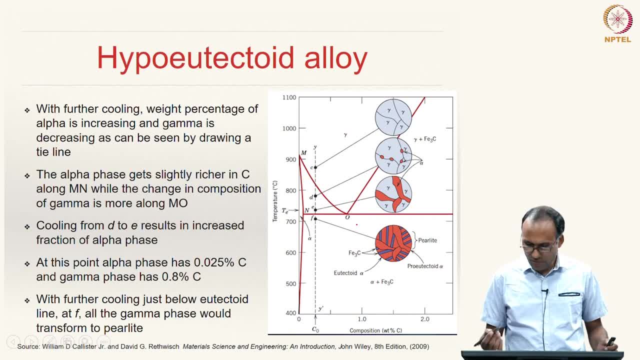 you reach point E, the weight fraction of alpha ferrite increases. As you can see, the red portions represents our ferrite and the weight fraction of ferrite has increased. And the moment it hits the eutectoid line, that is the NO line, then the remaining gamma. 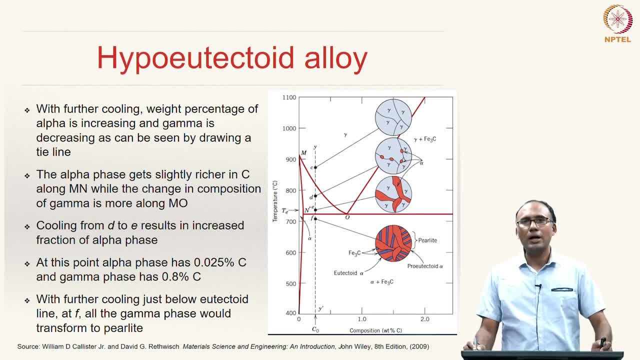 would have to undergo the eutectoid reaction and give gamma has to transform to eutectoid mixture of ferrite and cementite. And then you can see that eutectoid mixture of ferrite and cementite. here The blue one is cementite and the red one is ferrite. So you can see. 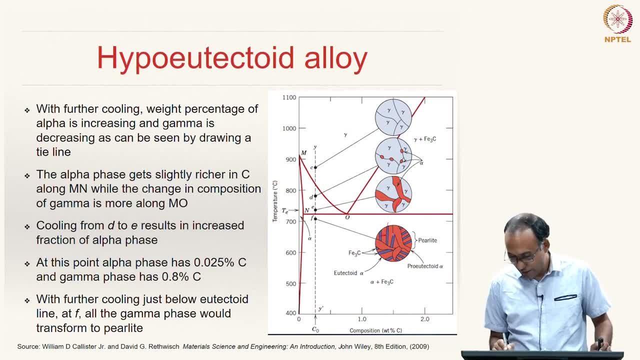 the thickness of perlite is…. In perlite, we know that the thickness of ferrite is little larger than thickness of the cementite, as we can see here, right, So this is the…. Now, this is our proeutectoid, So we can see. this is our proeutectoid, So we can see. 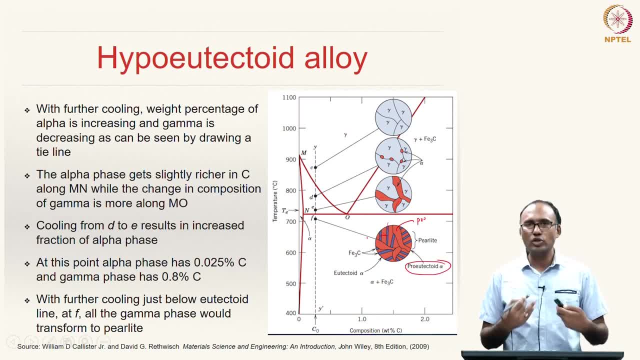 this is our proeutectoid ferrite, and the remaining is eutectoid mixture of ferrite and cementite. That is what is called perlite. alright, So in this region you have… Again, is this a single… This is a two-phase region, right, because you have ferrite and cementite. 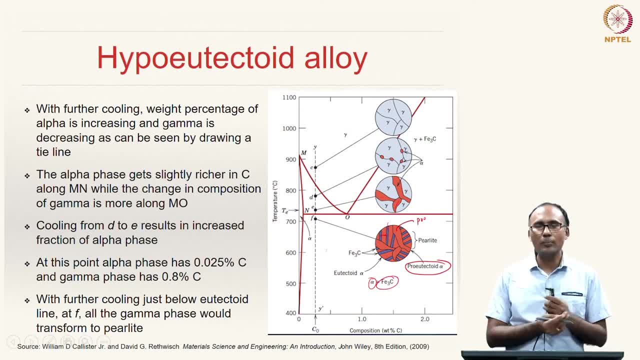 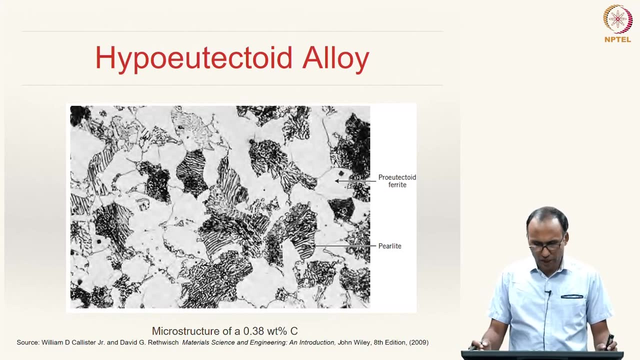 Again by drawing a tie line, you will know what is the composition of ferrite and what is the composition of cementite. total composition of ferrite and cementite. And so this is how the typical microstructure of a hypoeutectoid alloy of 0.38 percent carbon. 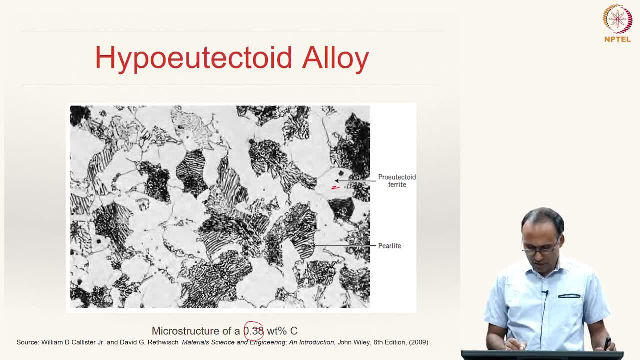 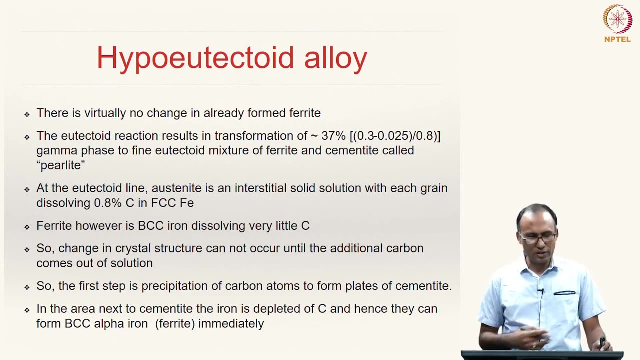 So you can see that this is proeutectoid ferrite and this is the alternate layers of ferrite and cementite called perlite. So you can see the eutectoid mixture of ferrite and cementite here. So we can see that with further cooling down, 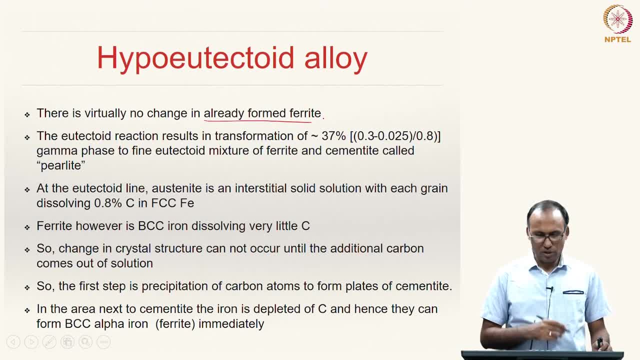 the virtually there is no change in already formed ferrite. So the eutectoid reaction results in the formation of about 37 percent. You can calculate the weight fractions from the tie line 35, 37 percent of gamma phase to fine eutectoid mixture of ferrite and cementite. 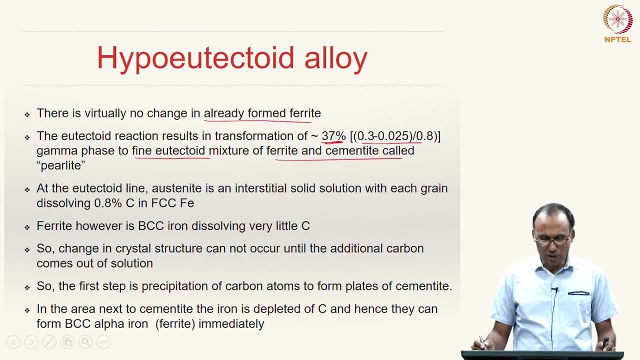 called perlite at the eutectoid line And at the eutectoid line. austenite is an interstitial solid solution, with each grain dissolving 0.8 percent carbon right At the eutectoid line. the austenite should be 0.8 percent carbon. That is what is we call eutectoid. 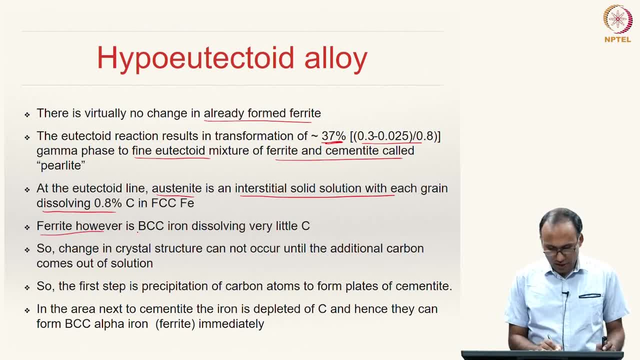 composition right And, however, the ferrite is a BCC iron dissolving very little C. So you have austenite, which is having 0.8 percent carbon, and it is transformed into ferrite and cementite, which is a C in. 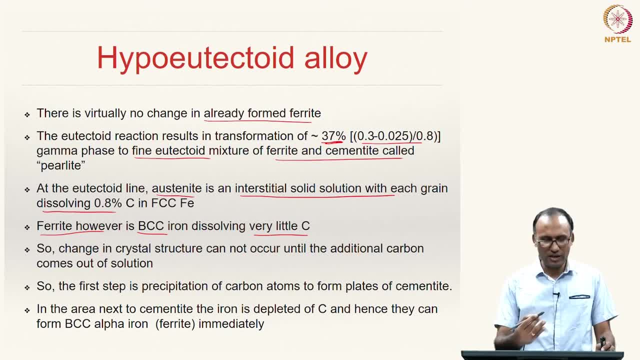 structure and it is transforming to a ferrite and cementite. and the ferrite is a BCC iron which dissolves very little C carbon. So the change in crystal structure cannot occur until the additional carbon that is sitting in austenite comes out of the solution right. 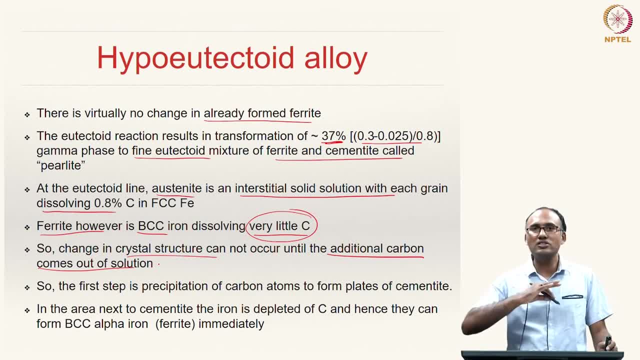 Because you need to provide sufficient time in order for this additional carbon to come out so that the alpha iron- so alpha iron- reaches its limited solubility. So the first step is the precipitation of carbon atoms to form plates of cementite. 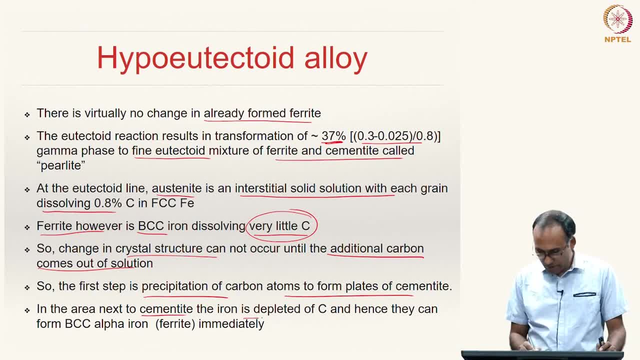 as we have already seen In the area next to cementite, the iron is depleted of carbon and hence they can form BCC, alpha iron- immediately, and that is how you will have alternate layers of ferrite and cementite. So this is the first step. So the first step is to form the 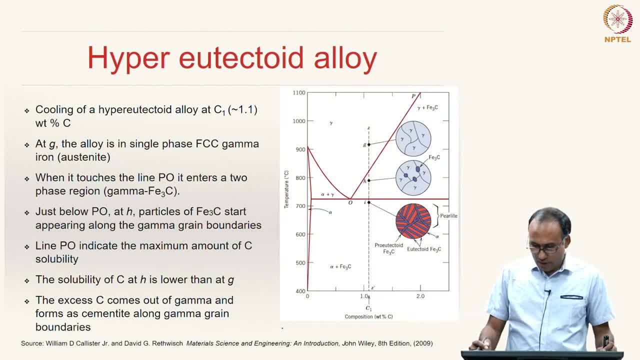 ferrite and cementite. Now let us look at hyper eutectoid steels Here. sorry, hyper eutectoid steels. Here we are looking at the alloy which has 1.1 percent weight percent carbon, Again at G. 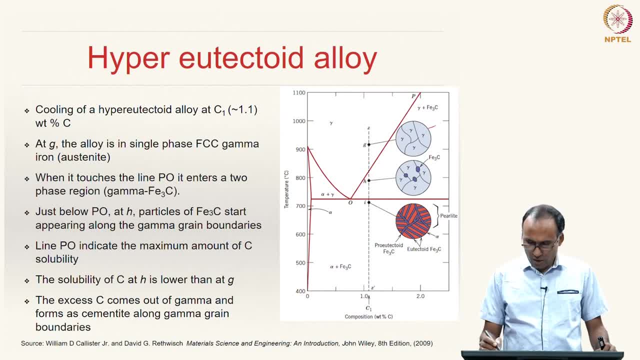 it is completely gamma iron and, as you are coming down, you will have pro eutectoid phase of cementite, because in this region, if you draw a tie line, to the left you have gamma and to the right you have Fe 3 C And hence the pro eutectoid phase will be of cementite. 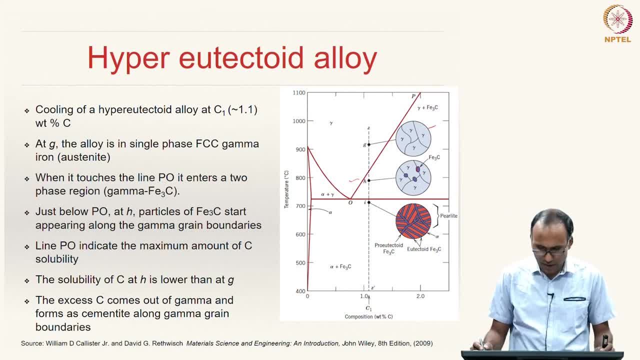 not of ferrite in the other as in, unlike in the other case, right. So for hyper eutectoid alloys, the pro eutectoid phase is cementite. For hyper eutectoid alloys, the pro eutectoid. 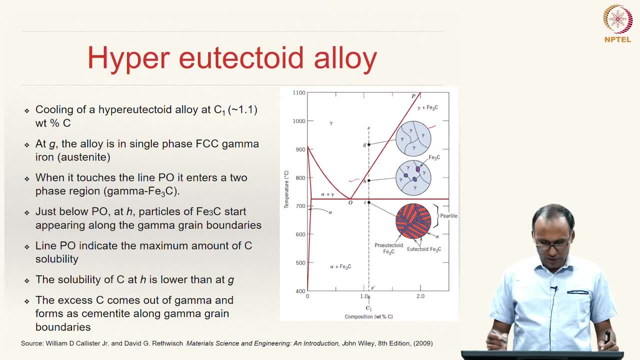 phase is ferrite, okay, So when the, when, the, when you are cooling it down, when it touches the line PO, that is, when it enters the two-phase region. Again, all the principles that we have adopted to calculate the composition of the two-phase region, that is, the two-phase region. So 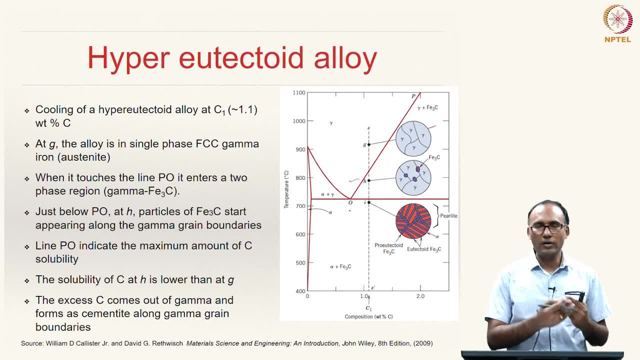 you can calculate the compositions and the weight fractions in two-phase region in the discussion of phase diagrams can again be applied here. right, So here the line PO sort of represents the maximum amount of carbon solubility in gamma. right, So the solubility. 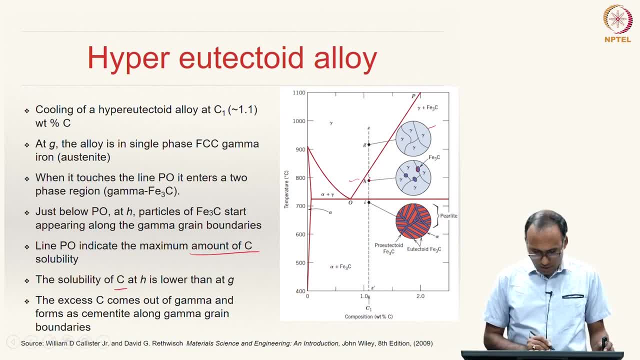 of carbon at H is lower than that at G. right At G you have this much solubility of carbon, So you would have 1 point 1 percent carbon By the time you commit. come to H, the solubility of carbon. 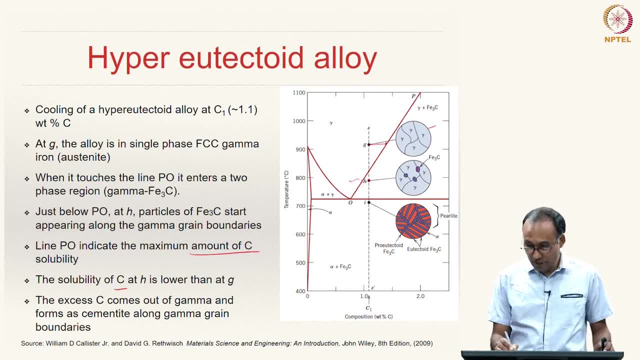 at this position is in gamma, for instance. in the gamma phase that is there, you have much less solubility, So this is the maximum solubility that is possible. So what happens? The excess C comes out of gamma, but it cannot come as pure C, but it should come out as. 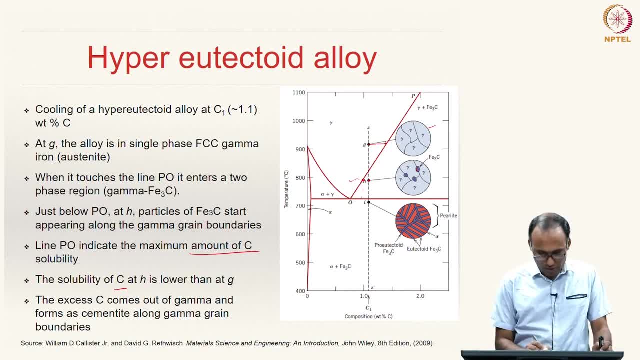 a solid solution. So it comes out as Fe 3C. It comes out as strictly as a solid solution. it comes out and the form of cementite along gamma grain boundaries. that is what we see. why it is come out as a grain boundaries because it has the gamma is already over saturated. 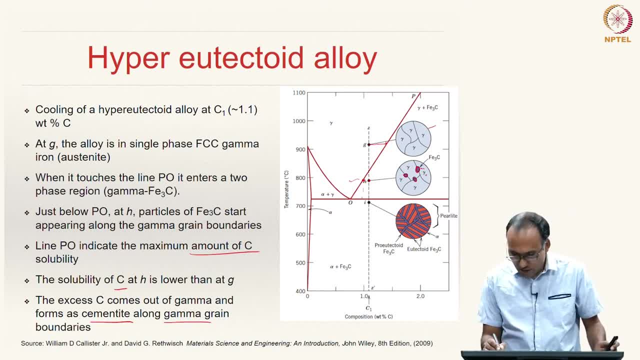 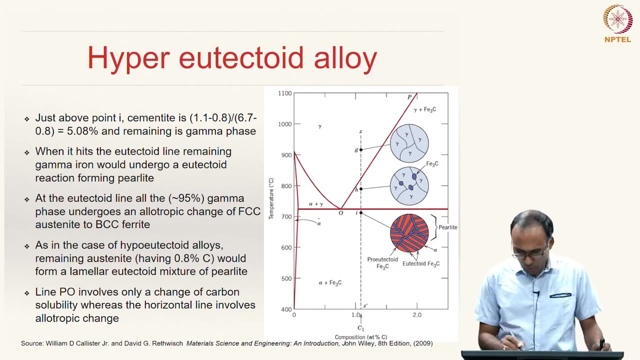 So, and hence it has to diffuse out additional carbon. that additional carbon comes and sits here as Fe 3 C here, whereas in hypotectoid steel it comes out as ferrite. So now just about point. I cementite is about 5 point, So 1 point 1 minus, So you can. 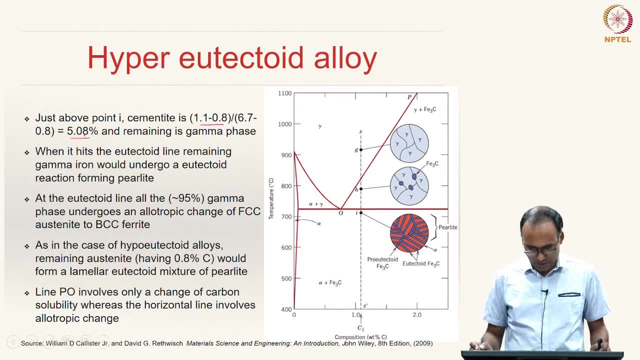 use the lever rule and then you see that it is about 5.08 percent and remaining is gamma. So there is only 5 percent cementite. all the remaining thing is gamma. So you have 5.08 percent pro eutectoid cementite, or 5, approximately 5 percent pro eutectoid cementite. 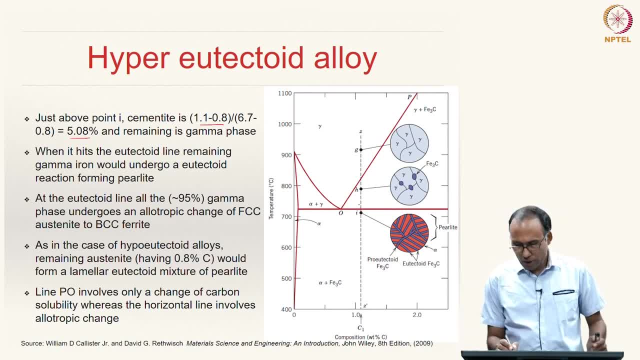 is formed and remaining 95 percent is still gamma. So when it is cross, cross, cross, So it is. So, crossing through this line at I, what happens? the remaining gamma, or austenite, will have to transform to eutectoid mixture of ferrite and cementite, So you will have 95 percent. 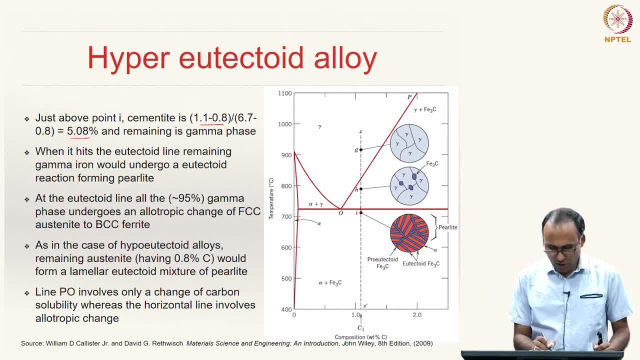 eutectoid mixture of ferrite and cementite or pearlite. So at the eutectoid line all the 95 percent gamma has to undergo an allotropic change of F, C, C austenite to B, C, C, ferrite, again right, and as in the case of hypo eutectoid alloys, the remaining austenite would form. 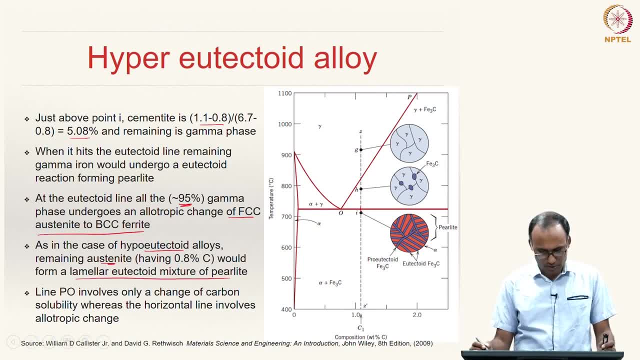 a lamellar eutectoid mixture of ferrite and cementite that is called pearlite. So please note that there is a difference in terms of the activity that is happening across line P? O and along the eutectoid line. So line P? O involves only a change of carbon solubility, that carbon is only diffusing out. 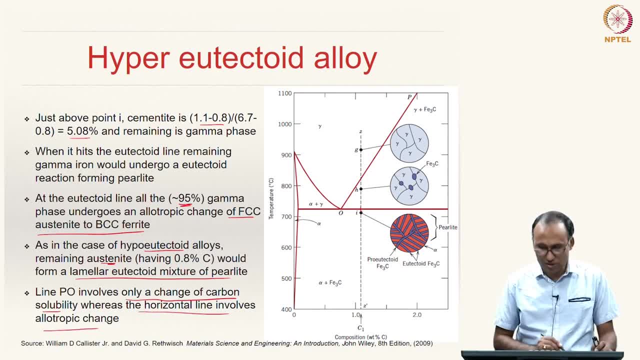 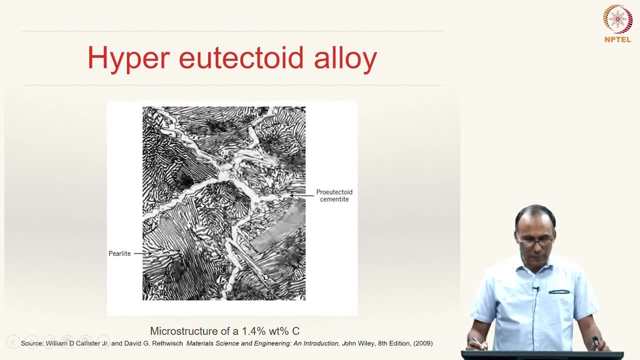 whereas the horizontal line involves an allotropic change. Here there is no allotropic change, but here there is an allotropic change that is taking place, and this is the typical microstructure of a hyper eutectoid alloy, wherein you can see. So it is discussed in this several times. 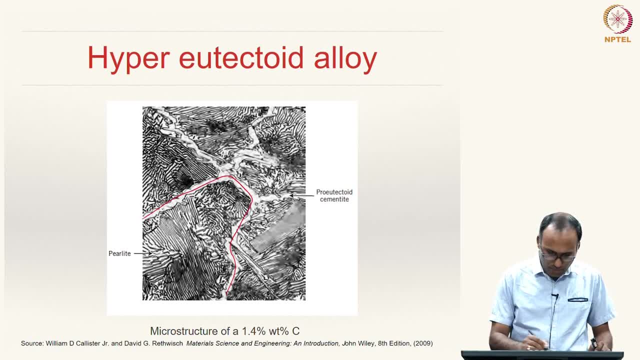 So let us take our mind and focus, the focus on this last step. So let us say: this is the. this white patch is our cementite, proeutectoid cementite that we have shown here, the proeutectoid cementite network, and this is all our alpha- sorry, not alpha. this is all our gamma. initially, 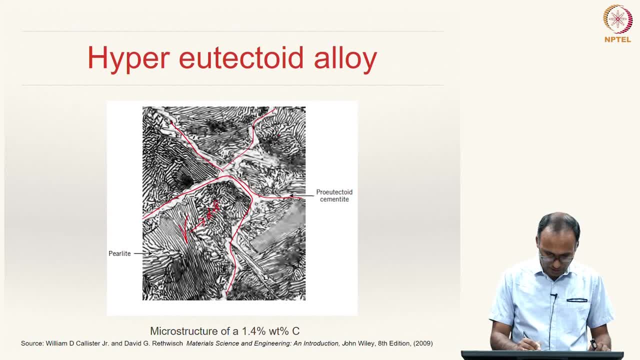 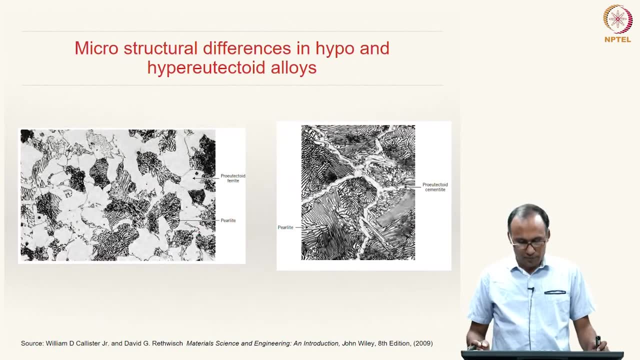 that has converted to pearlite alpha plus Fe 3 C, alternate layers of ferrite and cementite. So this is how the microstructure look like for a hypoeutectoid steel. this is the hypoeutectoid steel and this is your hypoeutectoid steel. So you can see that in hypoeutectoid steel. 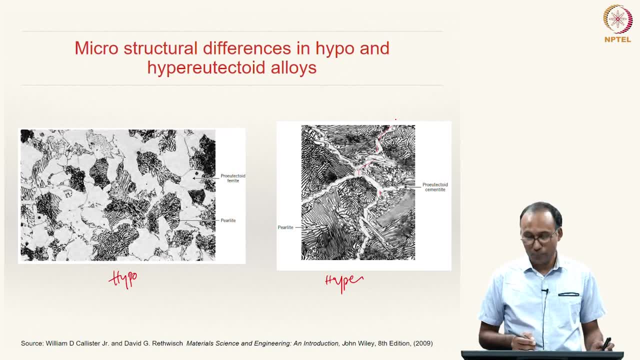 you have a continuous network of cementite throughout the microstructure, whereas here you have ferrite and proeutectoid, proeutectoid ferrite and pearlite. So the microstructures are very different for hypoeutectoid steels and hypoeutectoid steels, and we know that. 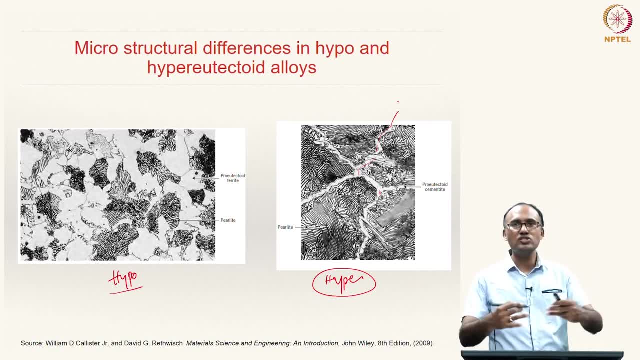 the cementite phase is brittle and hence the presence of continuous cementite network as a proeutectoid phase is something that one needs to be aware of. So this is what we are worried about as far as the mechanical properties are concerned of that system. So the mechanical effect on mechanical properties. the ferrite is soft. 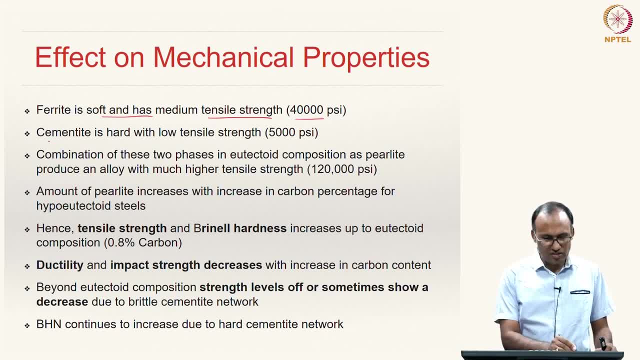 and has medium tensile strength, about 40000 psi, and cementite is hard with low tensile strength, about 5000 psi, And the combination of these two phases in eutectoid composition, as pearlite, produce a much higher tensile strength of an about 120000 psi. So as we increase the amount, 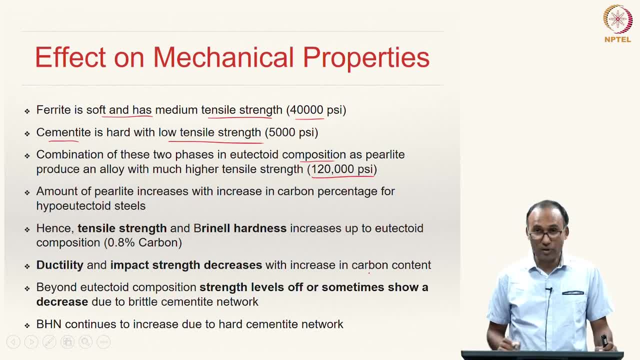 of pearlite. as we increase the carbon percentage for hypoeutectoid steels, amount of pearlite increases for, and hence the tensile strength and brinell hardness increases up to eutectoid composition, And ductility and impact strength decreases with increase in carbon content. 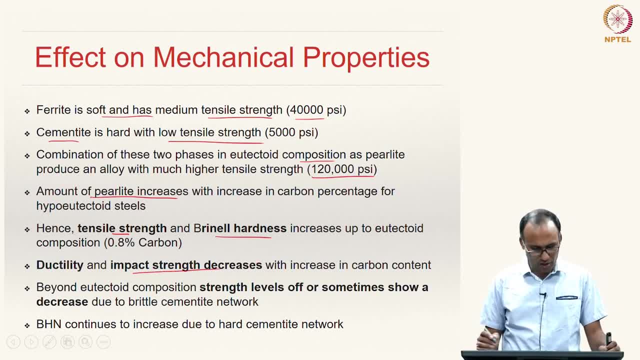 because carbon is going to increase the strength. So this is what we are worried about. So this is what we are worried about. So this is what we are worried about. So this is of hardness of the system or brittleness of the system and the beyond, the eutectoid. 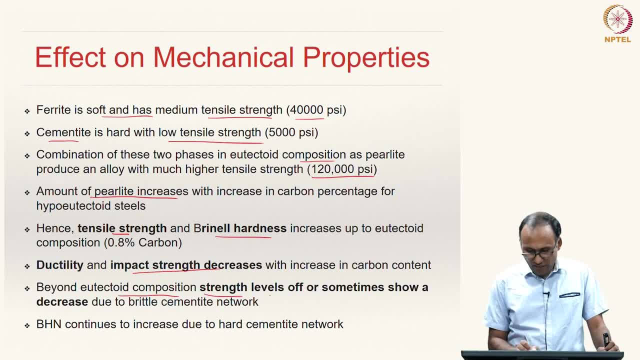 composition. However, the strength levels of are sometimes show a decrease due to brittle cementite network. that is what I said. hypoeutectoid steels are characterised by a continuous metal cementite network and that is going to limit the mechanical properties. then one could obtain, However, the brinell hardness number or general. 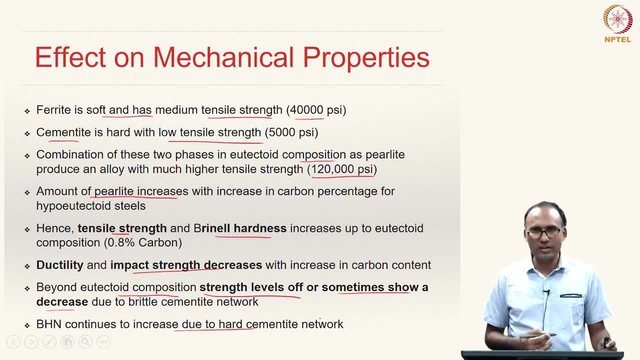 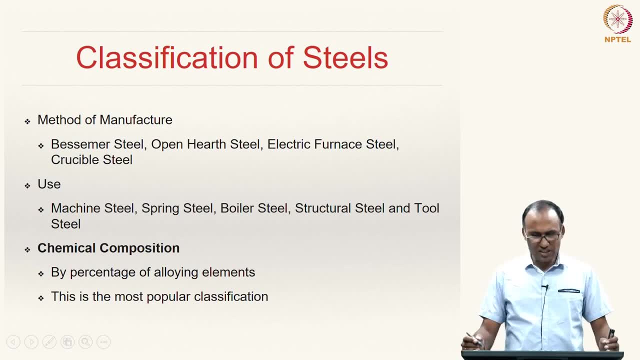 in general, hardness continues to increase due to hard cementite network increasing the fraction of the hard cementite Because of brinell hardness. these the component changes network. So now let us discuss about the classification of steels, how the steels are classified. The steels can be classified based on the: 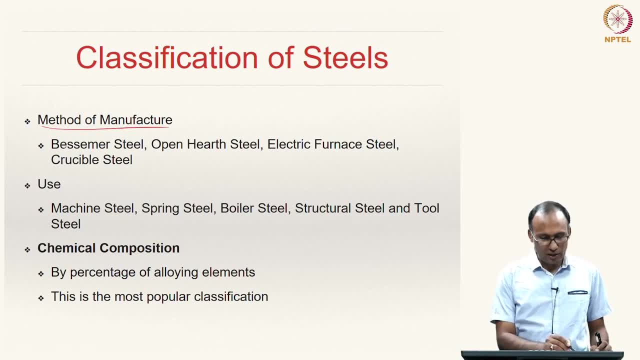 method of manufacture, the manufacturing process, So the depending upon if they are using bessemer converter to make steel, such a steel is called bessemer steel or open hearth steel, electric furnace steel or crucible steel, And sometimes they can also be classified based on the usage. 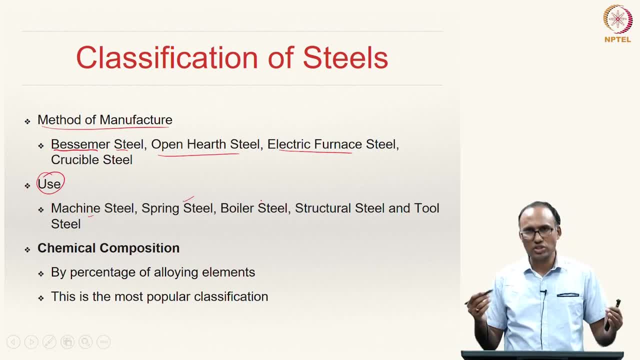 such as machine steel, spring steel, boiler steel, structural steel and tool steel. If you are using for tools, cutting tools and so on- then that such a steel is called tool steel. However, the most popular classification is based on the chemical composition, which 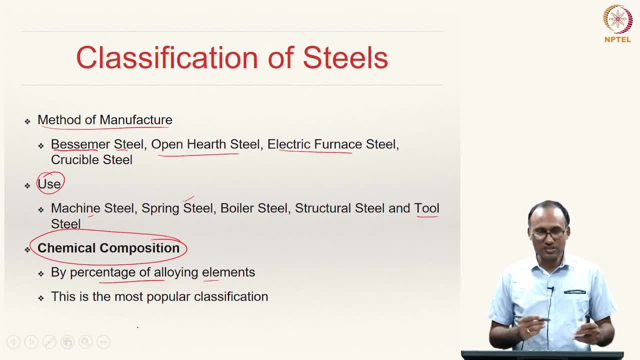 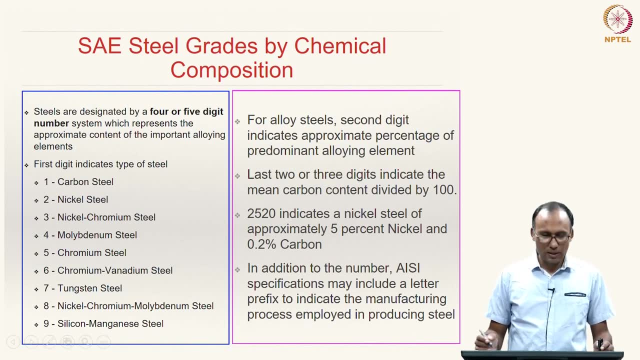 describes the percentage of alloying elements and that is most popular classification for the steels. So here in this class we will discuss the classification for SAE steel society of automotive engineering. The engineers have given some specifications for steel grades by their chemical composition. 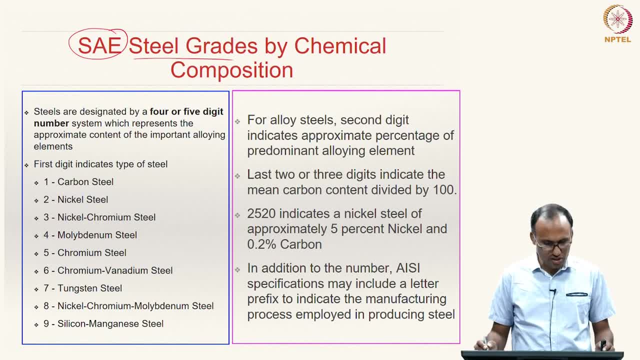 So usually, according to the SAE designation, the steels are designated by 4 or 5 digit number system which represents approximate content of the important alloying elements. So the first digit. so suppose you have 4 digits, this first digit represents that it 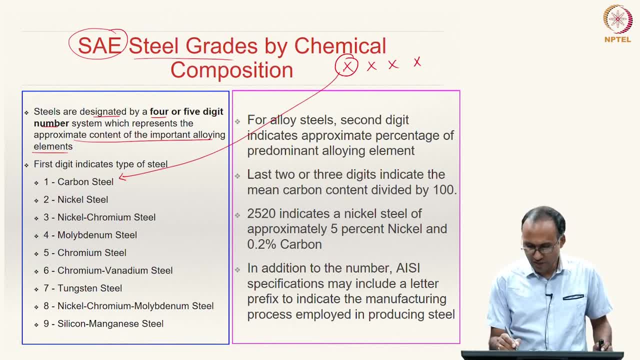 is carbon steel. If the first digit indicates the type of steel, then it is carbon steel. If it is 1,, then that is a plain carbon steel, And if it is 2, it is a nickel based steel. If it is 3, nickel chromium steel. If it is 4, molybdenum steel, That means primary alloying. 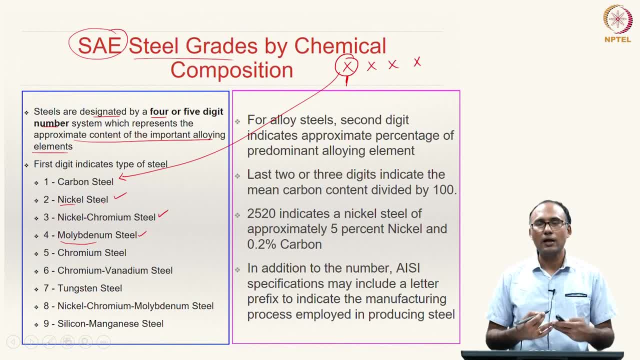 element is molybdenum. Here primary alloying element is nickel, like that. So here carbon means there are no other alloying elements, plain carbon steel. Except for some impurities it is only a plain carbon steel. So for alloy steels the second digit indicates approximate percentage of the predominant 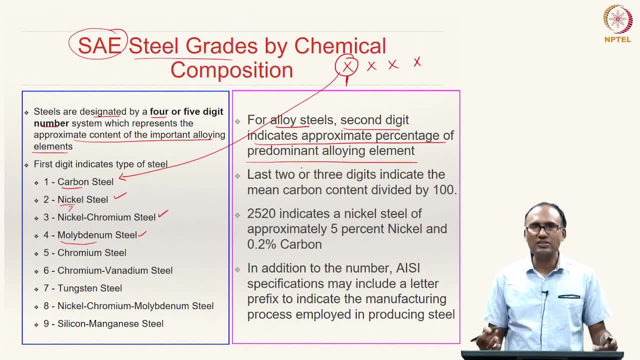 alloying element. So, for instance, if you are talking about nickel steel, the second digit represents approximate percentage of the nickel percentage in that steel And the last 2 digits- or 3 digits if it is a 5 index notation- represents indicate the mean carbon. 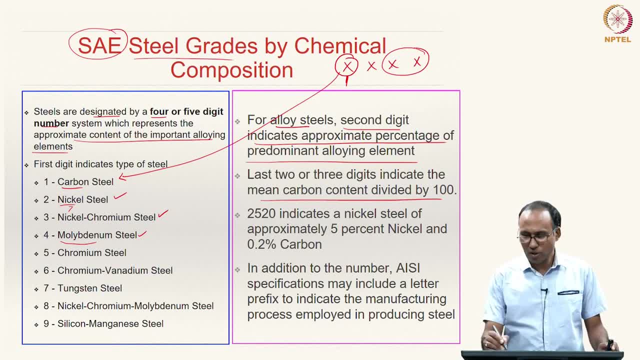 content divided by 100, right? So let us say, if it is 40, then that means 40 by 100, that is 0.45.. So for instance, if I take 252, 0 steel indicates, 2 means is a nickel based steel indicates. 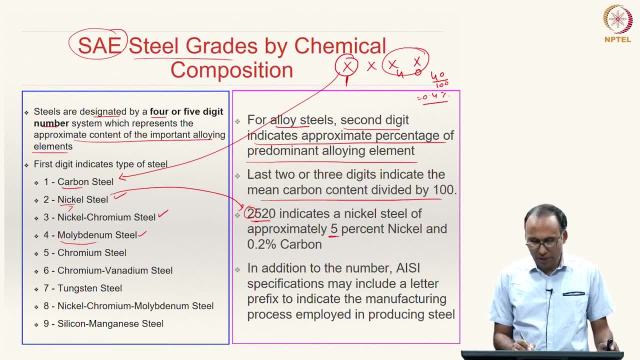 a 5 percent, approximately 5 percent nickel and 20 by 100 0.2 percent carbon. If I am talking about 1020 steel, that means is a plain carbon steel. There is no other alloying element and it is 0.2 percent carbon. That means it is hypo tactile steel. In addition, 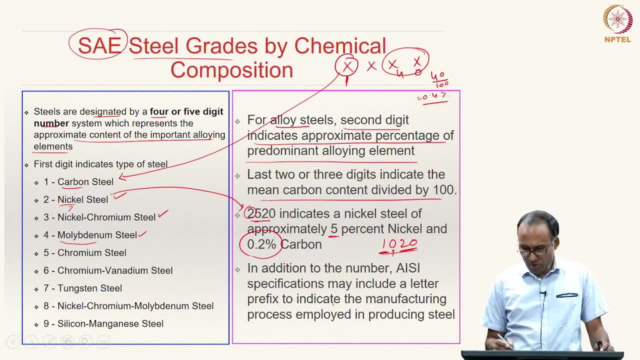 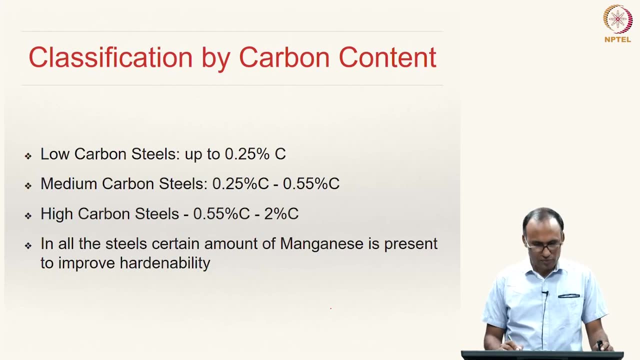 to the number. Sometimes the specification may also include a letter. For instance, if it is written E, that means it is electric furnace steel. So to represent the method of manufacturing, there will be a letter that is usually used before that. 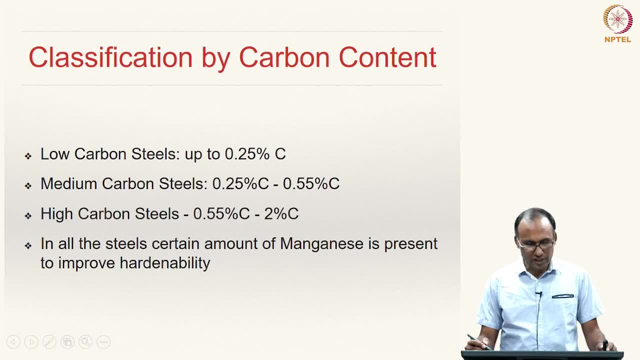 And again, the steels are classified based on the carbon content. If the carbon content is less than 0.25 percent, then such steels are called low carbon steels. If it is between 0.25 and 0.55, then it is medium carbon steel, And if it is between 0.55 and 2, high carbon. 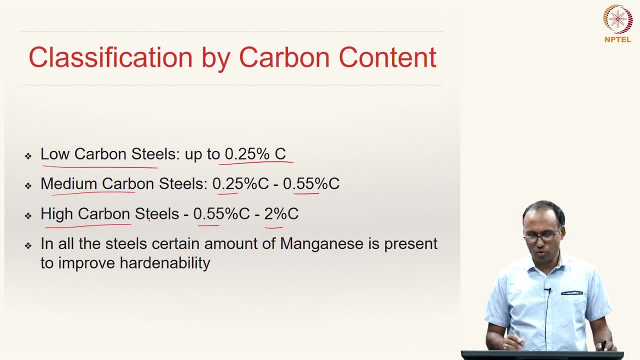 steel. So by that definition all hyper-eutectoid steels which are having carbon content point greater than 0.8 percent are high strength high carbon steels. And most of the hyper-eutectoid steels are low carbon steels or medium carbon steels, And some from 0.55 to 0.8 percent. 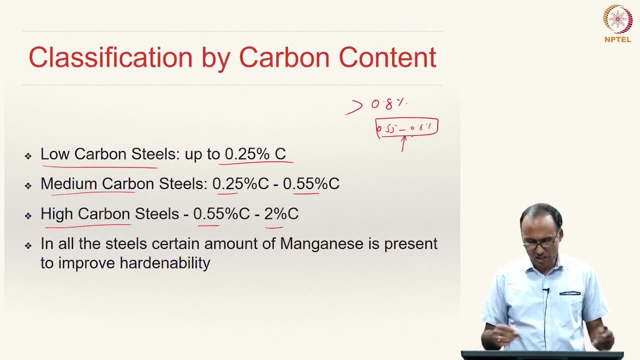 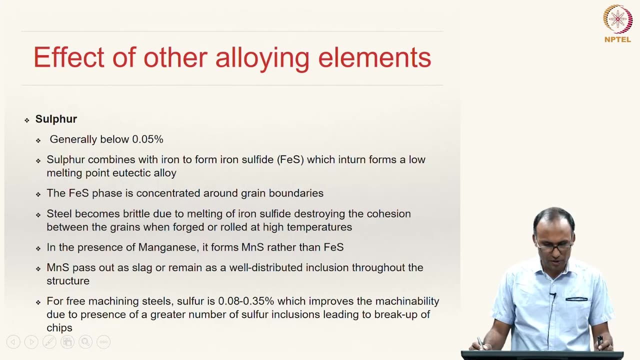 carbon. these steels, of these, of hyper-eutectoid steels, are high carbon steels And all the steels you always have certain amount of manganese because of the need for improving the hardenability of the steel, even for the plain carbon steel. Now let 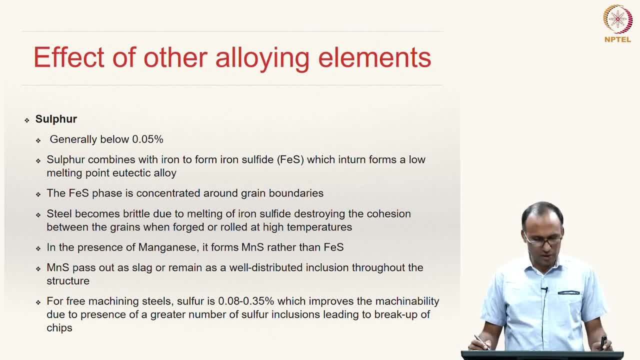 us look at effect of other elements on the properties of steels. So first let us look at the sulfur. Sulfur is generally maintained less than 0.05 percent in steel. What when it present in steel, the sulfur can break with iron to form iron sulfide, FeS, which in turn forms 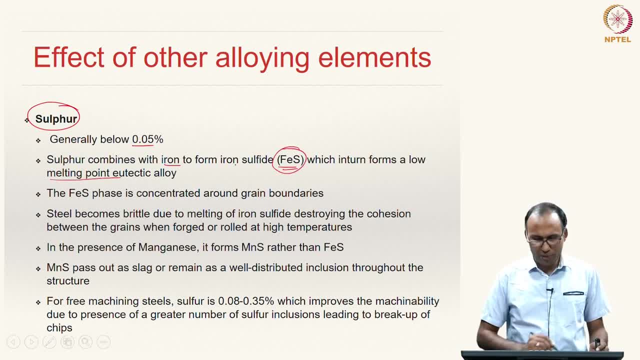 a low melting point eutectic alloy. So FeS is a low melting point eutectic alloy and this FeS phase is usually concentrated around the grain boundaries And steel sometimes becomes brittle due to melting of iron sulfide. because it is a low 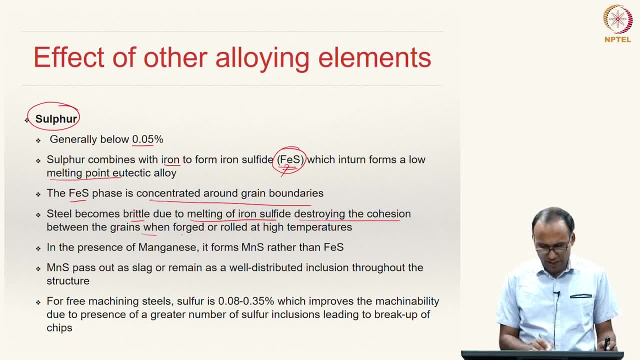 melting point, eutectic phase and destroying the cohesion between the grains when it is used at or or an early temperature. So and5 attempt wide brown at 2300, 0.5 percent и 0.8 percent rest actually loose around 2. Peel in the coal form with 6ほど. only It has. 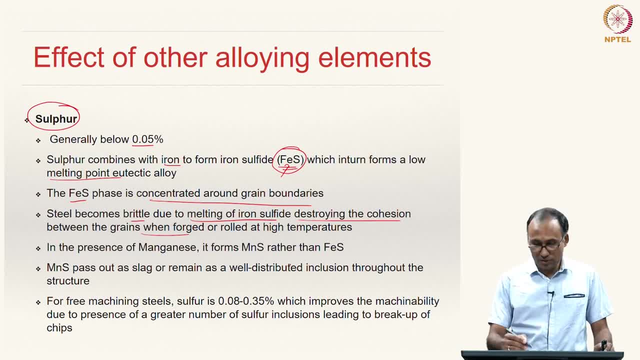 high temperature. So, and hence the sulphur presence in iron around iron atmosphere is not actually good. However, if, as we have discussed always, this plain carbon steel will have some amount of manganese, However, in the presence of manganese, it prefers to. 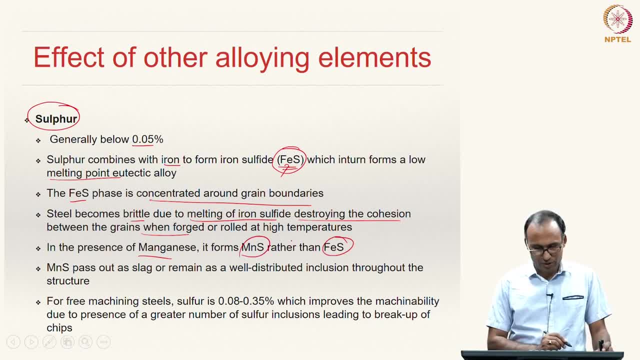 form manganese sulphate rather than ferrous sulphate, And the manganese sulphate actually has an advantage. It actually manganese sulphate passes out as slag or remain as a well distributed inclusion throughout the structure without causing the adverse effects that ferrous sulphate would cause, And for free machining steels, sulphur is usually. 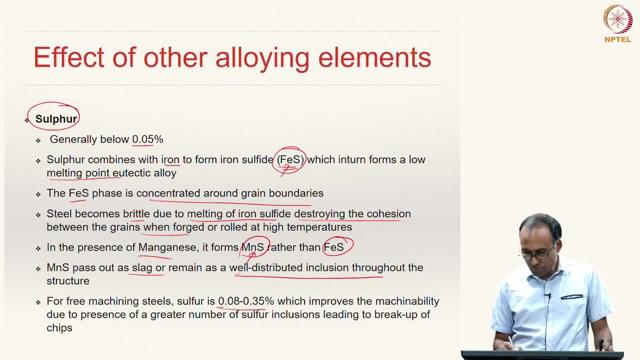 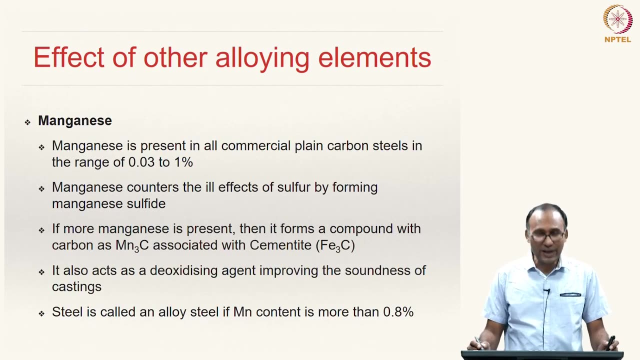 maintained at 0.08 to 0.35 percent, which improves the machinability due to the presence of greater number of sulphur inclusions, leading to breakup of chips, because it is giving mass, So it is giving additional hardness and it allows us to break the chips better. Manganese. 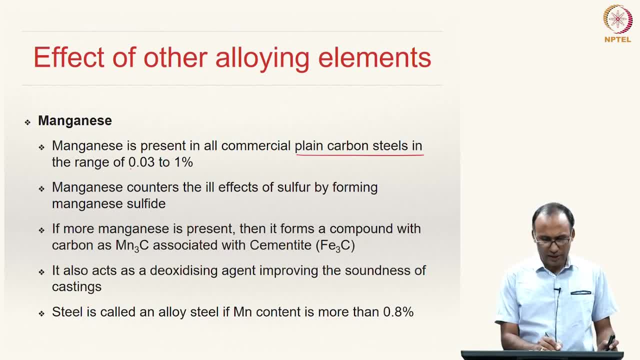 as we have discussed, is present in all commercial plain carbon steels in the range of 0.03 to 1 percent. So one of the major advantages of manganese is that it counters the ill effects of sulphur by forming manganese sulphate. However, if more manganese is present, then it forms 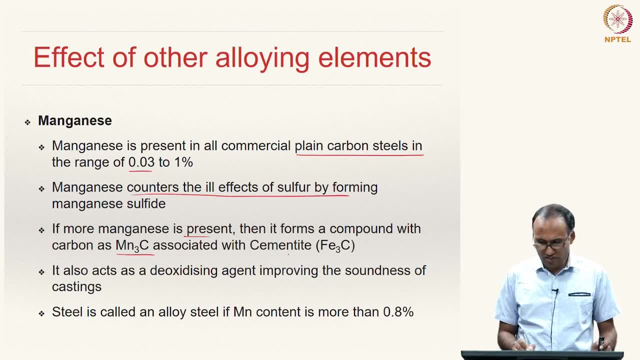 a compound with carbon, as Mn3C, associated with cementate Like Fe3C, is formed. similarly you will have Mn3C And it also manganese also acts as a deoxidizing agent, improving the soundness of casting, So it will get rid of some gases that are probably trapped in the liquid state. Steel is called. 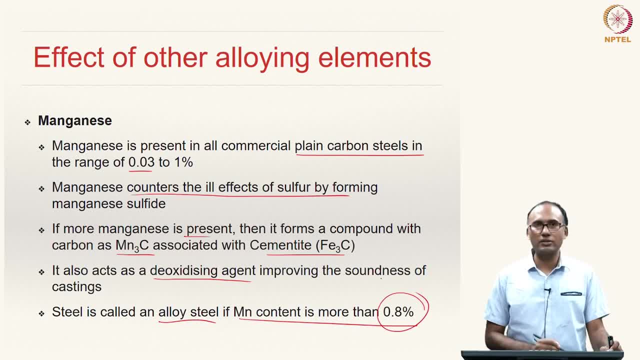 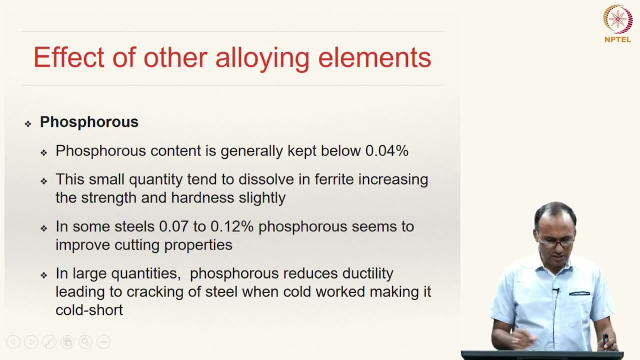 an alloy steel if manganese content is more than 0.8 percent. Otherwise it is called plain carbon steel, And the next alloying element that we are interested in is phosphorous, So phosphorous content is usually kept very low, less than. 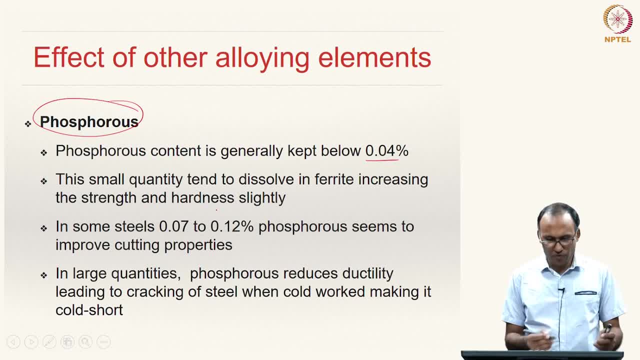 0.04 percent, And the small quantity of manganese is usually kept very low, less than 0.04 percent, And the small quantity of manganese is usually kept very low, less than 0.04 percent. And the small quantity of this small quantity of phosphorous tend to dissolve in ferrite, increasing. 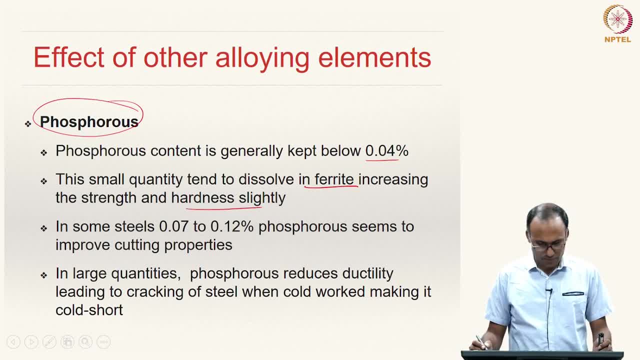 the strength and hardness of the steel slightly. In some steels you may have a higher percentage of phosphorous in order to improve the cutting properties. However, in large quantities, if you have large quantities of phosphorous, it reduces the ductility, leading to cracking. 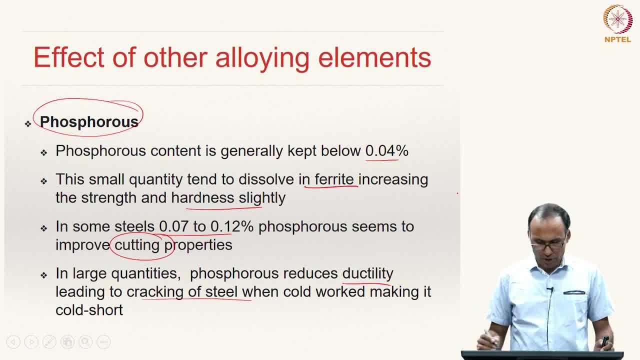